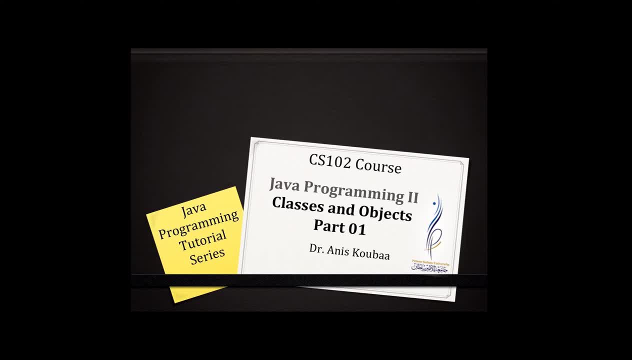 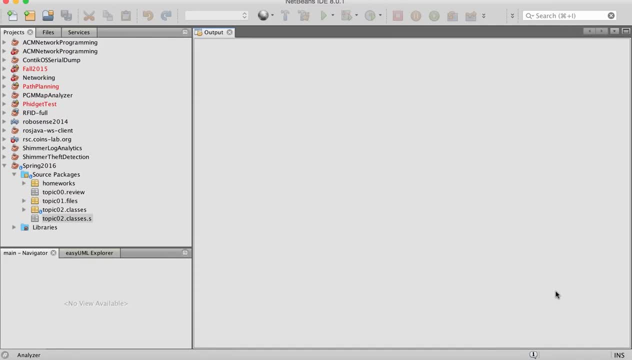 Okay, so as I mentioned, today the objective is to learn about classes. You will understand why classes are important and how to declare them. So in order to understand this, I'm going to start from a very basic program. I would like to create a student program. 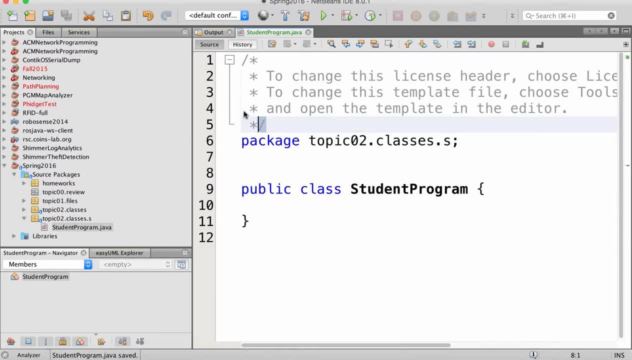 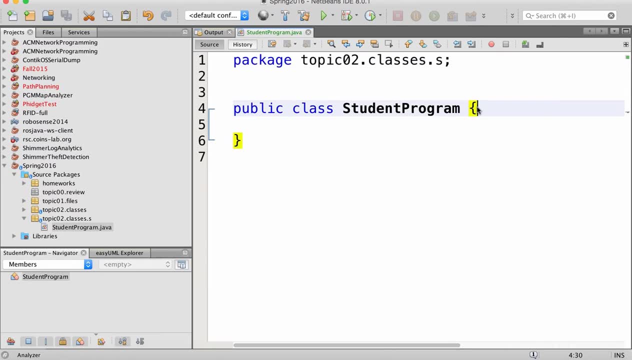 A very simple class. So in this program, what I would like to do is to create two students and print their information. 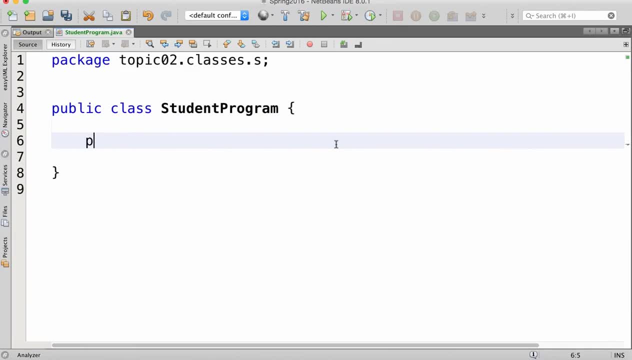 Of course, as you do in CS101, you declare public static void main string args. And now we are ready to write our program. This is. 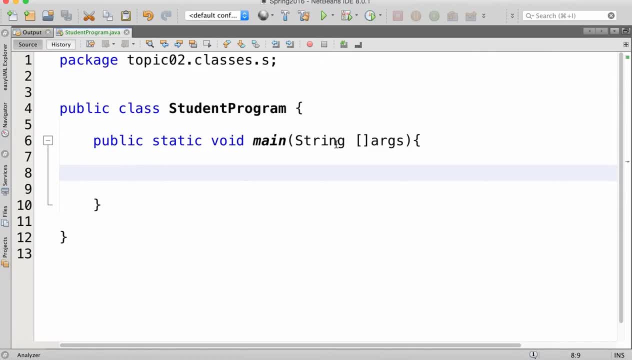 Using just the CS101 concept. So now if you are asked to create two students, for example, with their first name, last name, and mobile phone number, and GPA, and display their information, how are you going to do it? So tell me. 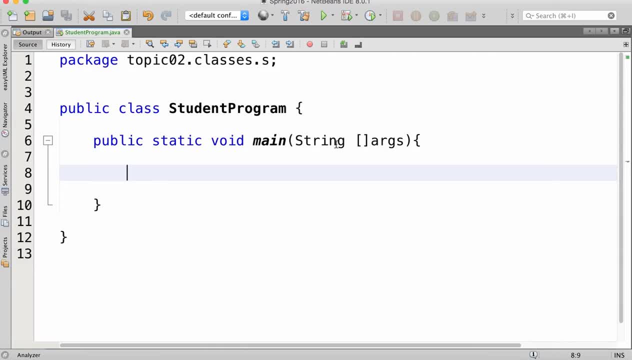 Yeah, but now we have to create something. Declare what? The name? The name. Why? The array? We don't need array now. We need to create variables to put the names. Okay? 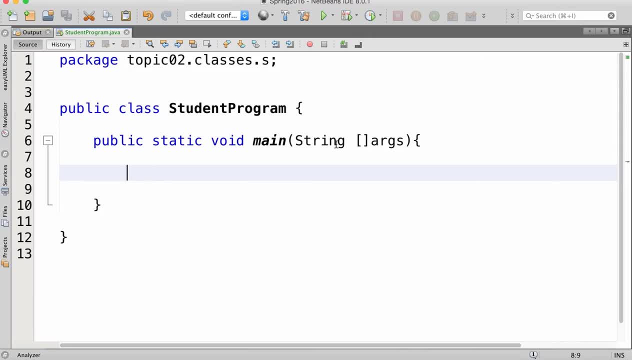 So the array, if we have a sequence of things to store. Okay, it's true that we have two students, but two students is not necessary to create an array for them. I want just to create two students or even one student. 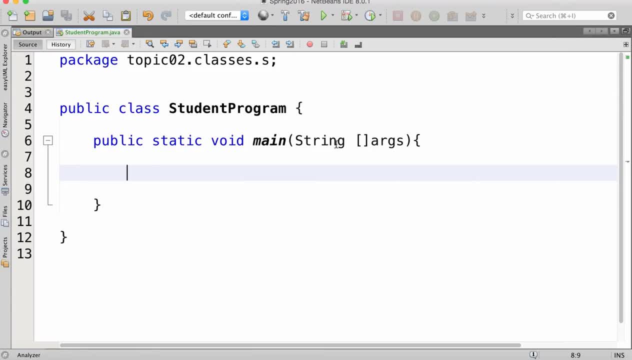 So what I should do? For the names or... String. Okay, so string, yes. 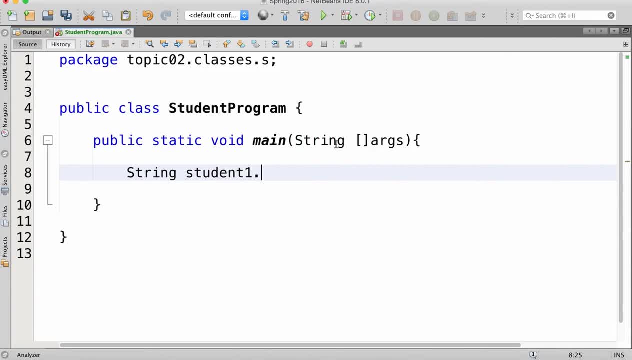 Okay, let's call it student1.student1.firstName. Okay, and I will give it a certain value. And for the last name. 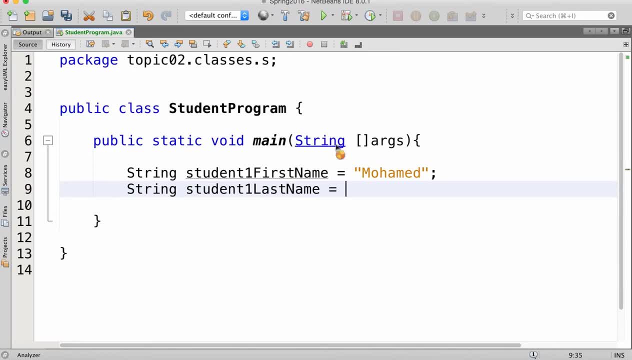 Okay, student1.lastName.equal. Okay. Okay. 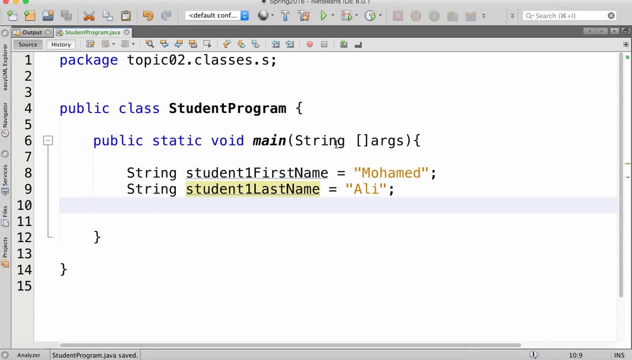 I would like to define a phone number. I'm going to define it as a string because if you make int the zero at the left side is not going to be stored. 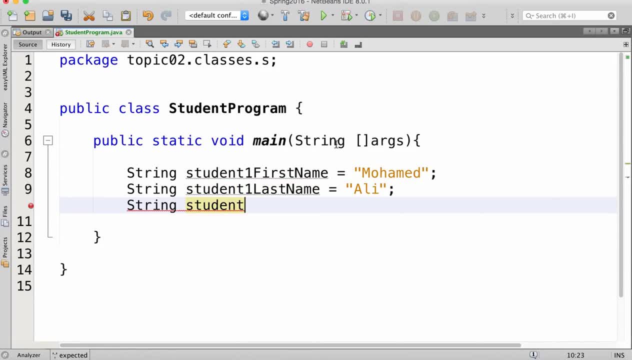 So this is student1.phone. Okay, I'm going to give any number. And let's say GPA. 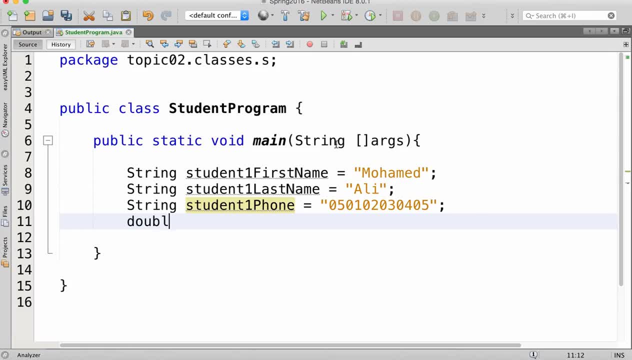 So how do you define the GPA? Okay, I'm going to define it as a double. 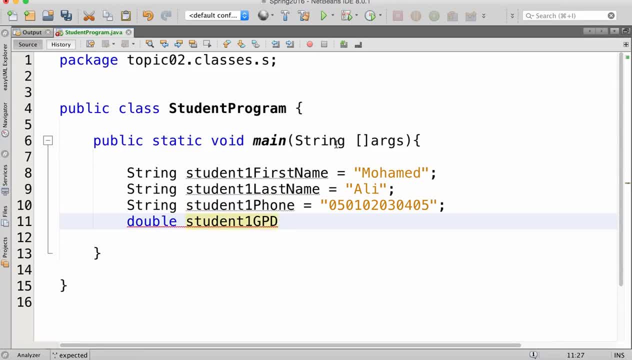 Student1.GPA.equal to 3.3, for example. 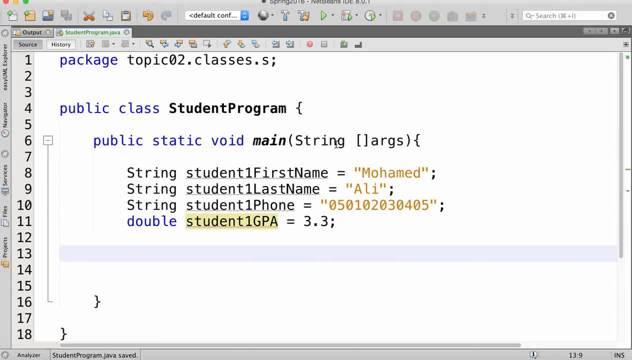 So now if I want to define a second student. Yeah, I need to copy all of this, right? And replace 1 by 2. And then, for example, changing the different values. 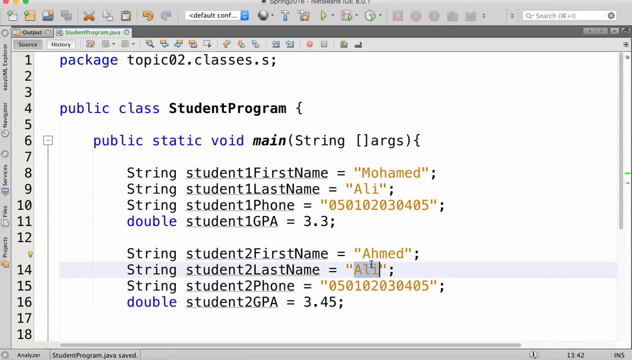 Okay. I'm going to put some values. Change the number. Okay. 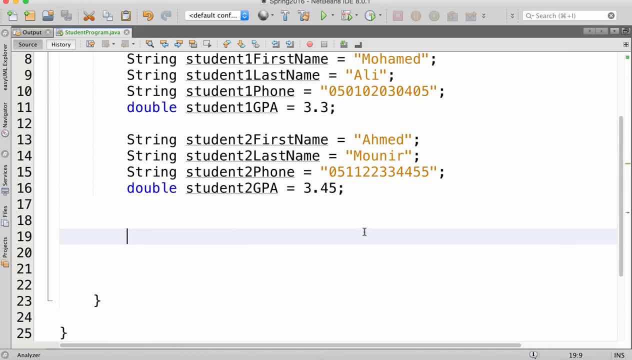 It seems to work. And then if I want to display, we can do system.out.println. Okay. 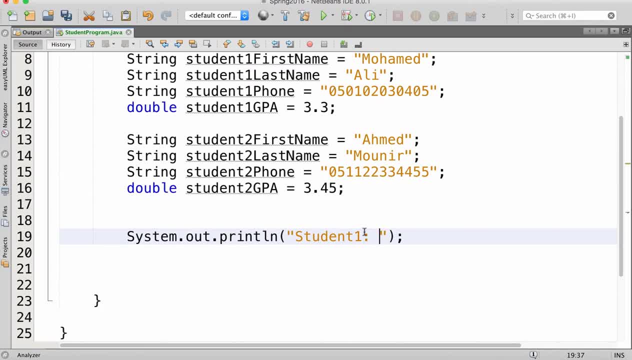 sout, for example, student1. And I will make an sout. First name. Last name. I will copy this. 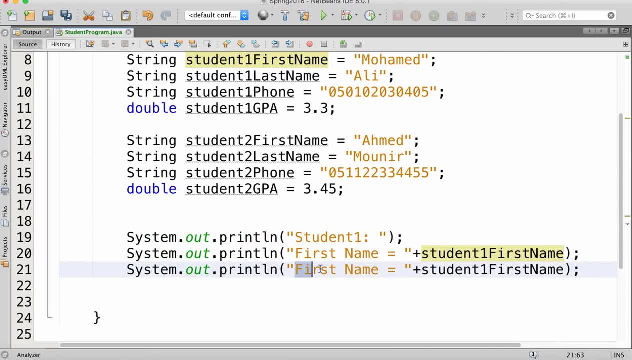 I will do the same for last name. And I will do the same for... And I will do the same for... Last name. Last name. 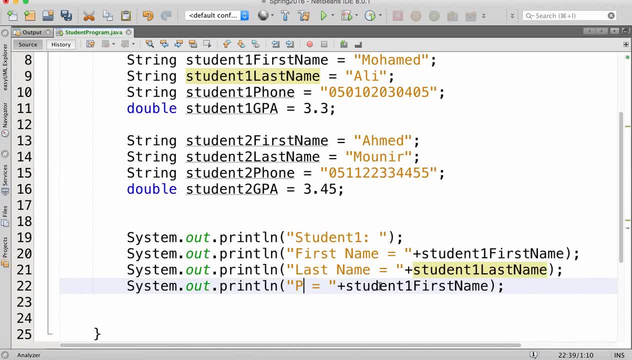 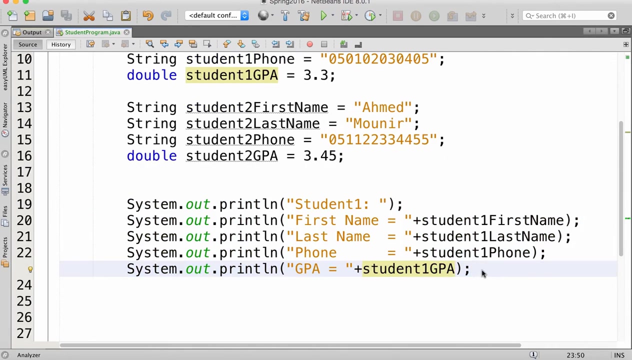 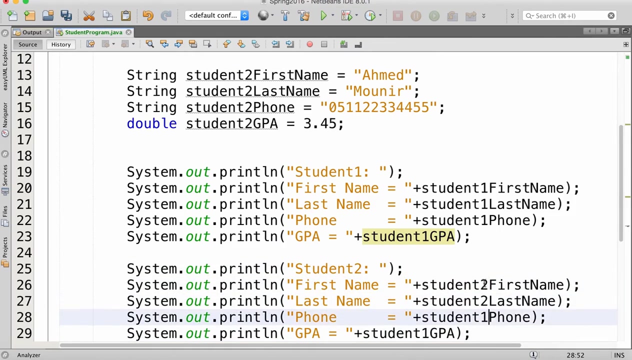 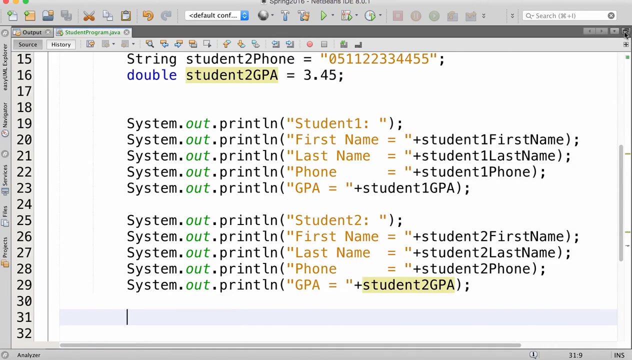 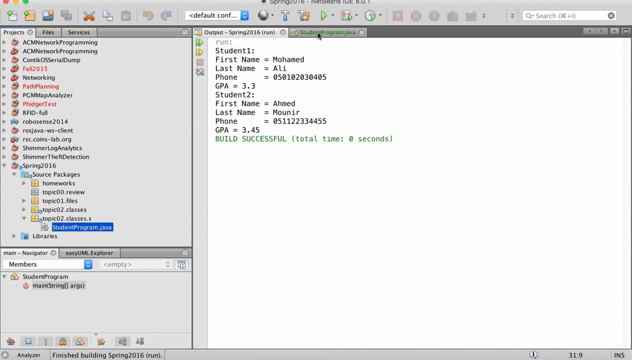 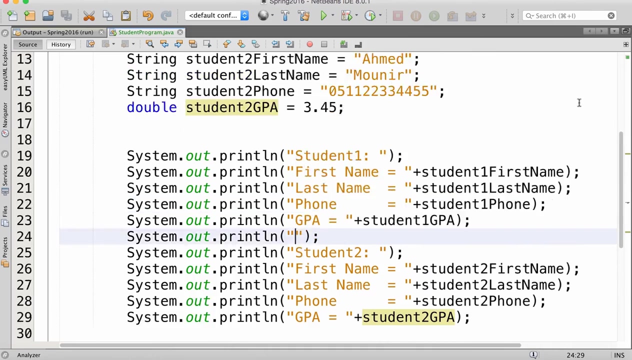 for what phone so student one phone and I will do the same also for the GPA right student one GPA if I want to display for student to copy this make to first name okay this is to here to here and to here and here we have to so now let's execute so I did a correct program I can just add probably an S out here to have another space so my problem is correct right it does the work but the programming style is it good why no this is what you know already do you know 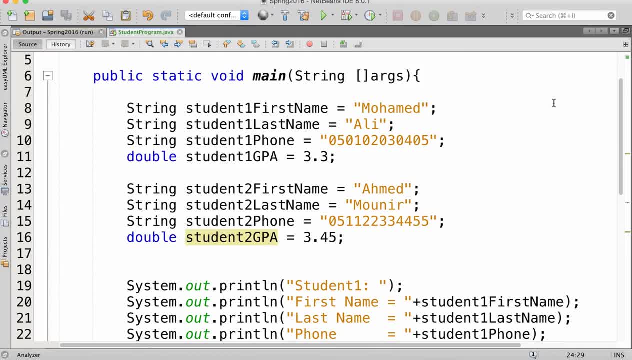 better things do you know a better way to do this okay this is one we are going to learn but in CS 101 do you know something that will reduce the code size if you are going to add a third student no loops if you are okay if I make a loop how what the loop will do for me nothing no I don't want to enter in the keyboard I want just to define them like this so is there anything in CS 101 that allows you to add a third student to the class if you want to you to reduce the code size no so now you will know how to reduce the code size using classes so what what do we observe here what is the observation we observe that there are common 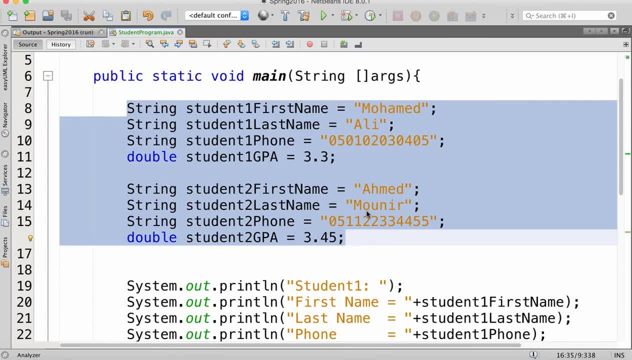 things right first student has first name second one has first name so there are a common thing so we can see that this can be seen as an entity that define define a student and also this one defines another student 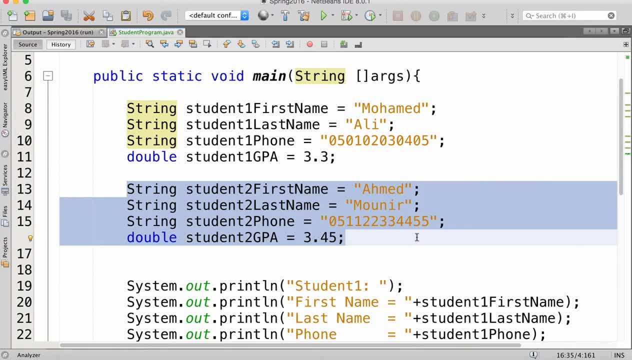 okay it will be good if you can put all together into some model into some structure and then use 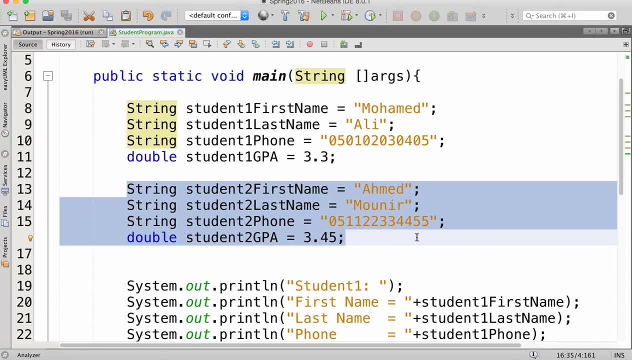 this structure to create to create these values right so this model or this structure in Java it's called the class we can define a class okay to put together a set of 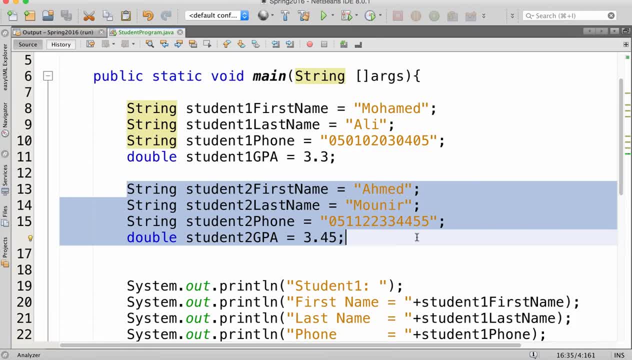 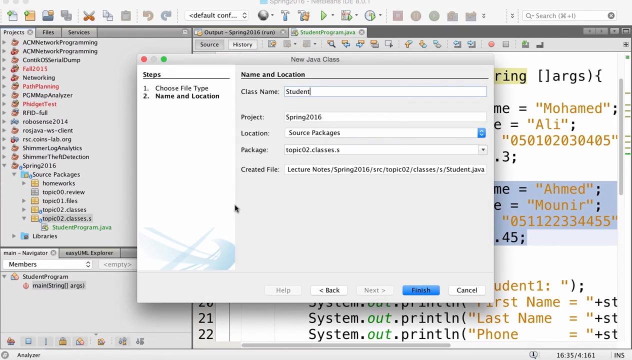 attributes we call them attributes like first name last name phone so all of these are attributes of an entity of a model of student okay that I can define so now the next question is how to define a class and the second question is how a class will be efficient in reducing this code size this is what we would like to understand Sahra okay so now I'm going to define my model or my class so I'm going to create a new Java class now which I'm going to call it student because this will represent a student entity a model for a student a representation of a student it's something like let's say abstract okay 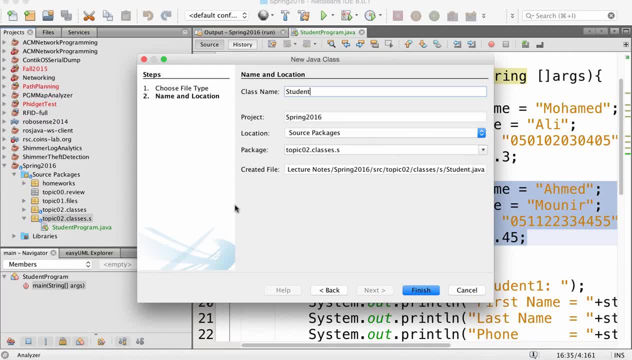 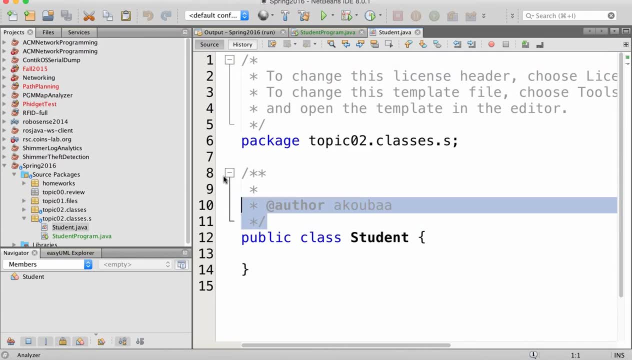 that give me an understanding of what is a student and what is not a student is through what through the attributes that defines the class so this is the class student I can also call it an entity class so here I define the class student you define the class student and then the next step is to define the 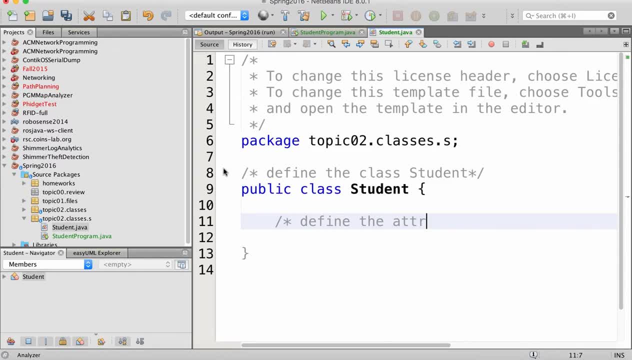 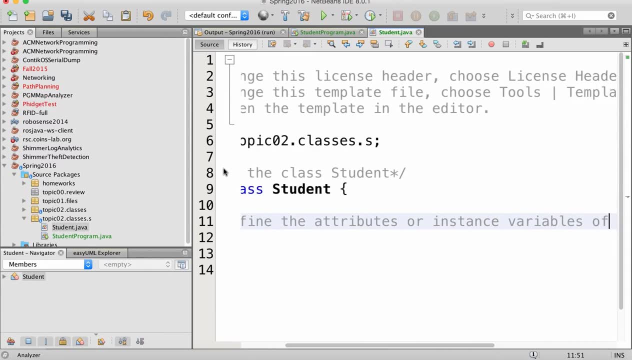 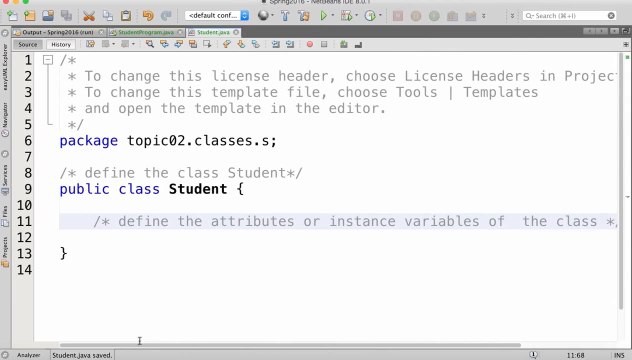 the attributes or also we call them instance variables of the class I think you know now what are the attributes of this class what are the attributes of this class 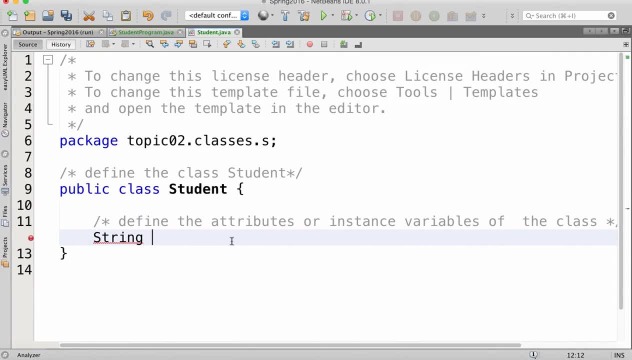 ok so I'm going to call it stream I don't need to write student one or student two because this is a model and later on you will see how we can use this model in our test program so I'm going to make first name as a first attribute ok and then I have a second attribute is last name so there is a convention when you write the attribute or the instance variable is that when it is composed of several words the first one is lowercase the second word start with a capital letter so this is a convention that you have to follow and I'm going to define another thing for phone and a double for the GPA ok so now this is a class I have everything that I need so the class is composed of two different things 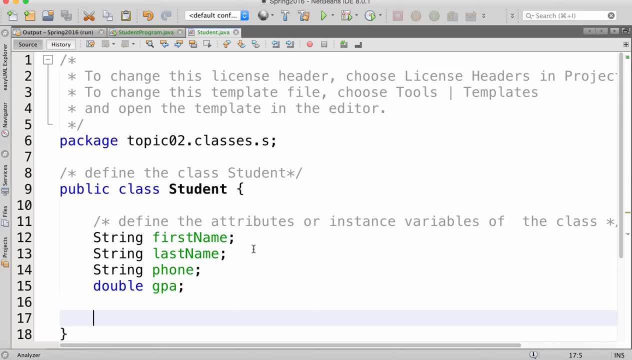 the first thing is our attributes this is what we have defined the second thing I'm going to talk to you about 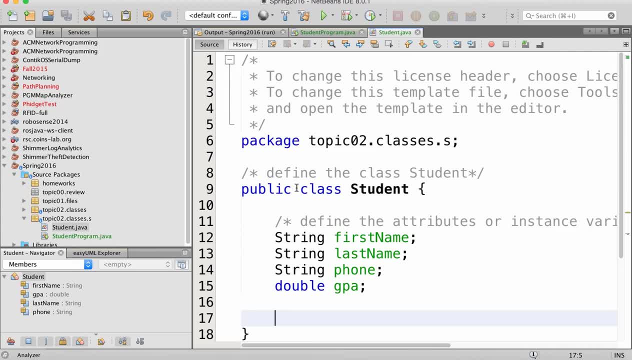 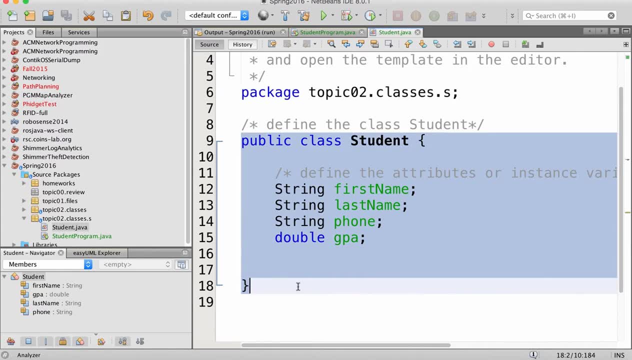 just in a moment but now let me see how this would improve the structure of my code so not this class doesn't contain a main function I did not define any main and this is something new with respect to what what you have seen in CS 101 because usually do either a main function or you define other methods or other functions on the top so here we didn't define any method we didn't define any function we just defined some instance variables 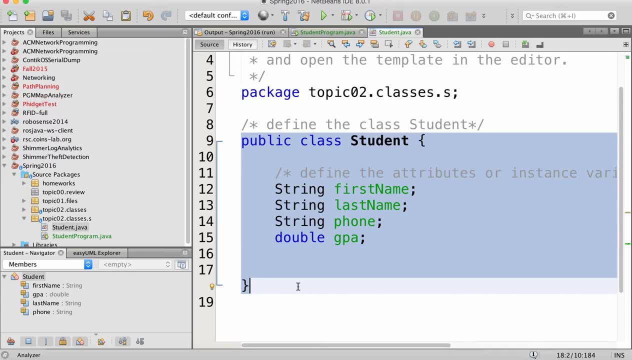 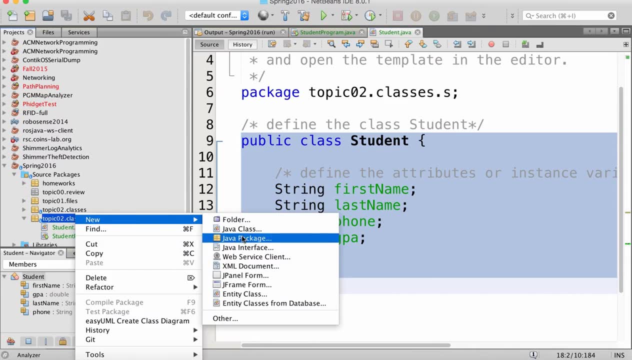 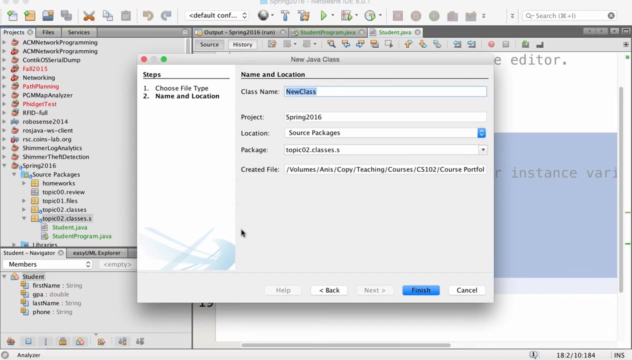 this variables are properties of the class they are attributes of the class they characterize the plus so how this helps I'm going to create another class so usually we create the entity class or the model class as a separate class it doesn't have any method or any my any main method and then I'm going to create something to test so this is where my program is going to run I'm going to create the application now and 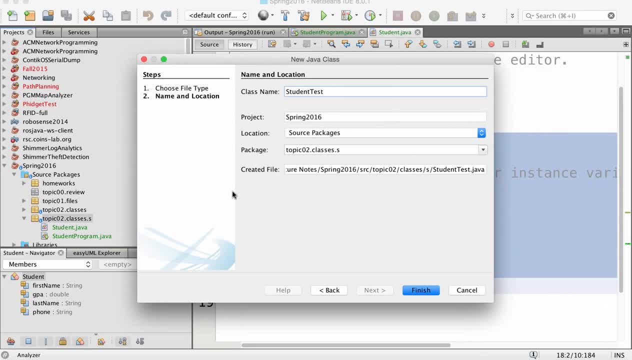 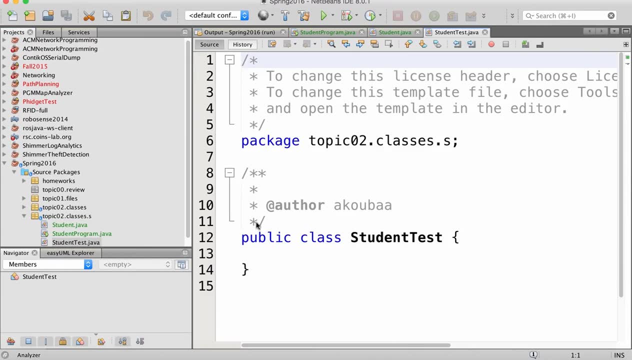 this application will use the model that I have created the model student in order to create new variables of type student so students is going to be defined as a new type and 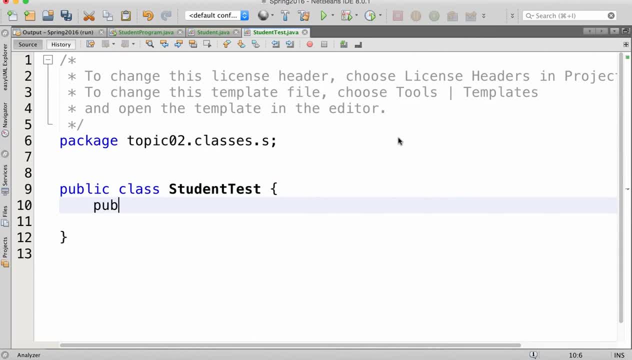 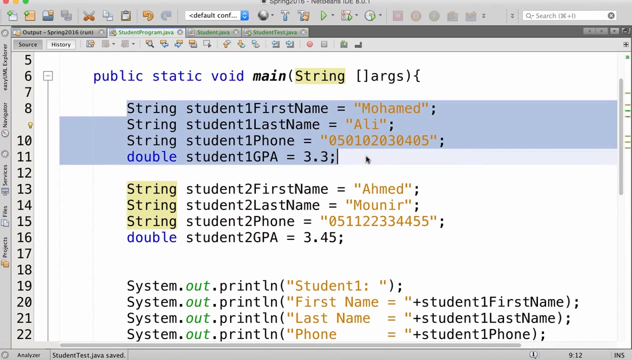 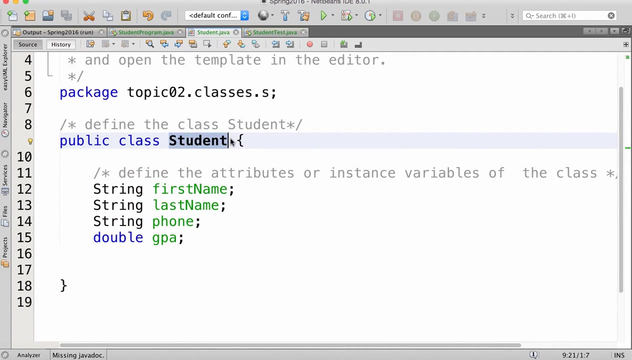 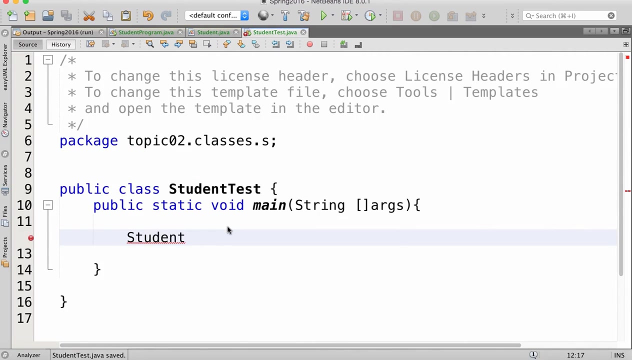 here this is a test class I'm going to define public static void main okay and now I would like to do the same thing here I don't need to define variable by variable okay this this way is if I don't use classes which is not efficient as we have agreed now I have a class student and this class defines a new type for me so I can use this type in order to declare a new variable student student one okay so student 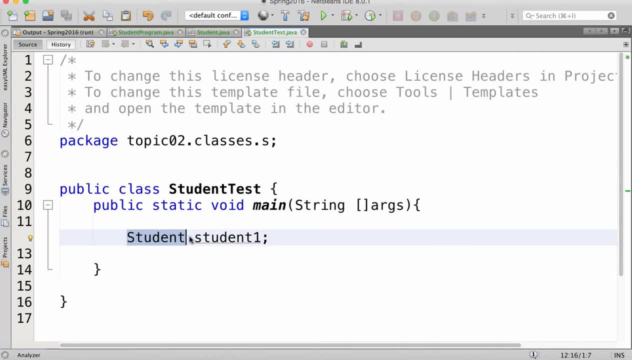 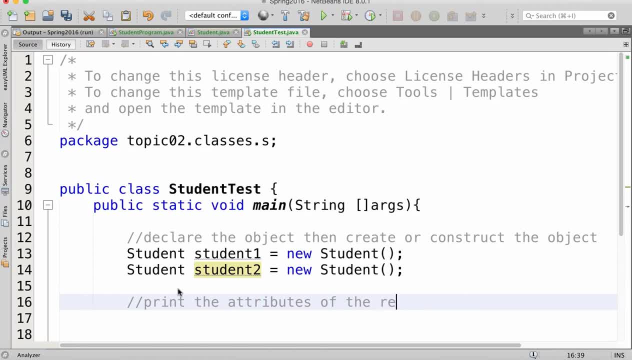 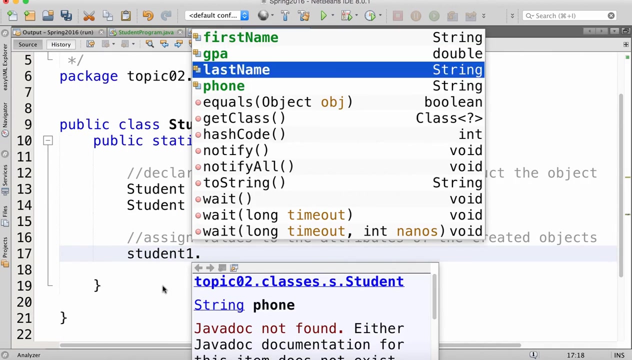 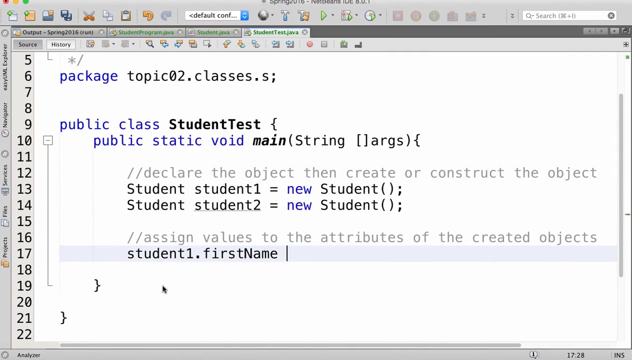 of the created or before printing assign values to the attributes of the object so how can I do this now when we didn't use object we defined independent variables now we have a structure we have a structure for example student one is a structure it contains some properties if I click dot I'm going to have access to all the properties defined in that structure in that class or in that object so I can do now first name equal Muhammad student one dot last name equal honey okay student 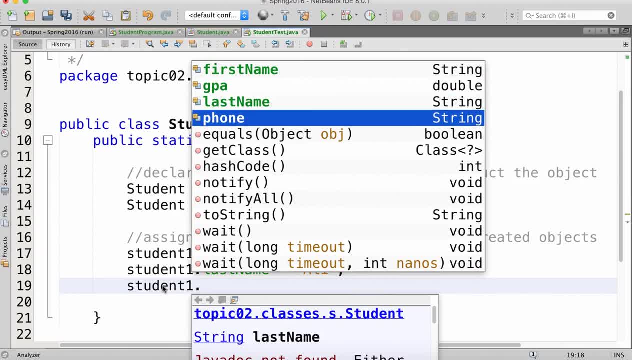 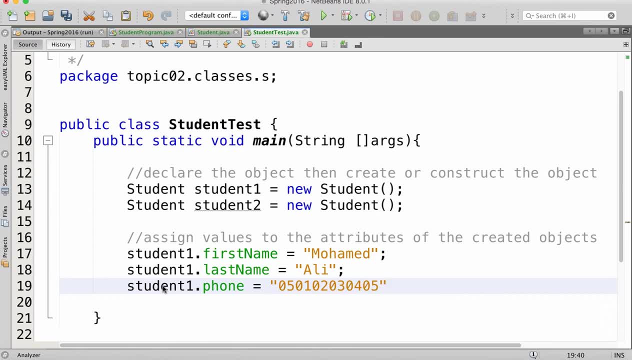 one dot four equal zero five zero one zero two zero three zero five and finally student one dot GPA equal to three 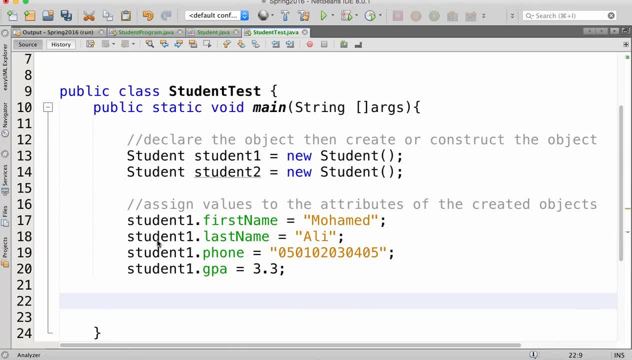 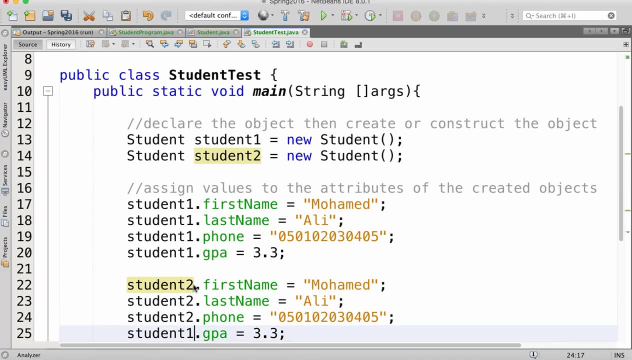 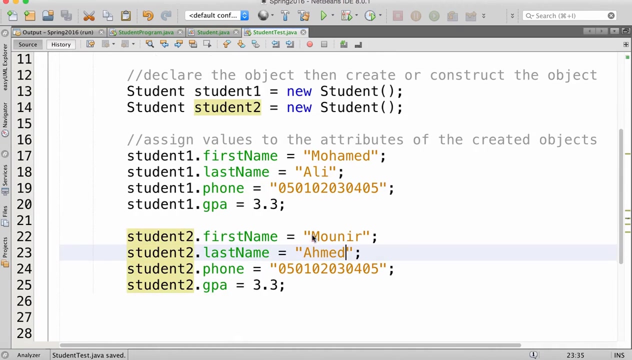 dot three likewise I will do the same but for student two so here I'm going to assign the value okay and here zero five one one two three four five five and let me change the GPA so what's better now we have one step of improvement it's only one step you'll see more improvements later 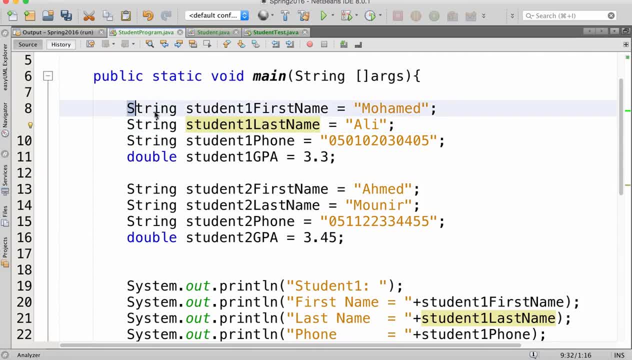 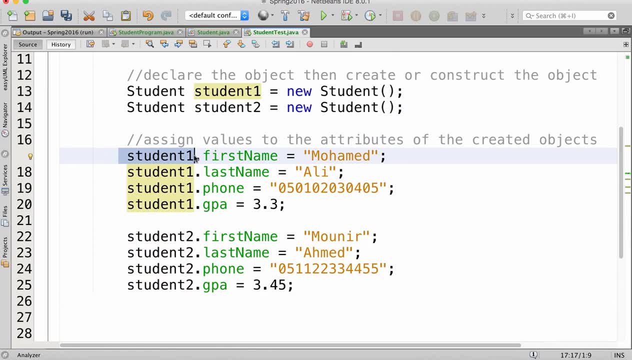 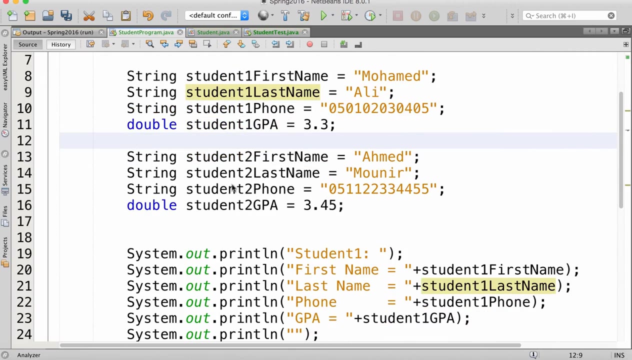 instead of having independent variables like you see here we are having a new variable we are having variables that are related to objects so at least in terms of organization that is much better so hello okay it's much better now imagine that I have a new attribute to add if I want to add for example the address if I am at this case I have to create two variables one others for student one and one others 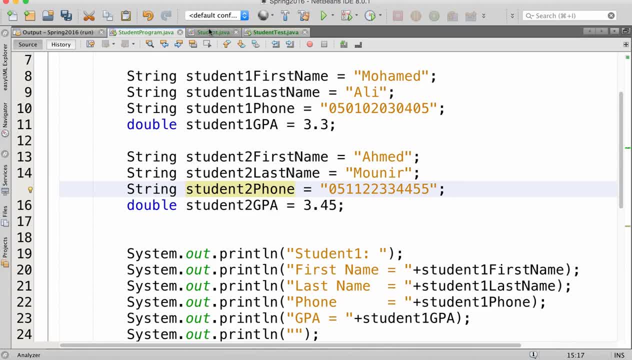 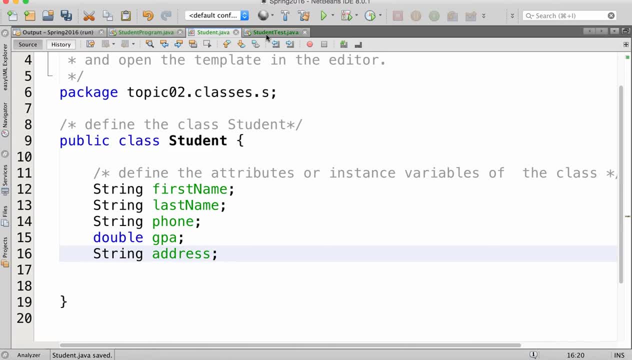 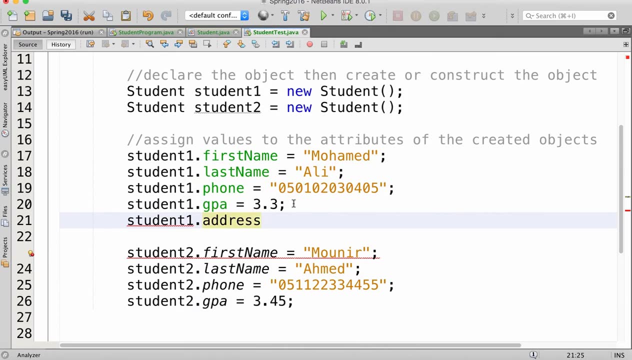 for student two I I don't need to do the same okay I need just to define it in the class and then with some magic if I make student one I'm going to find the address attribute defined okay so let me put real here okay 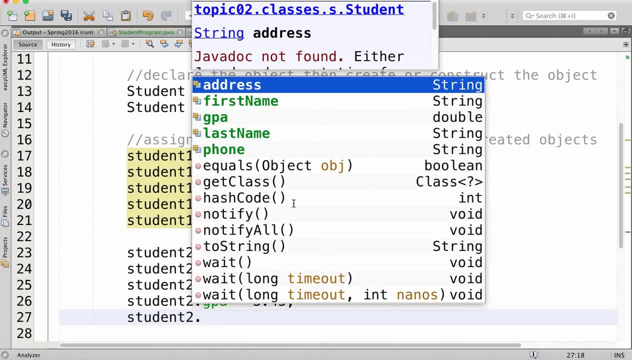 same for the class and then with some magic if I make student one I'm going to find the address attribute defined okay so let me put real here okay so let me for student two I have also an address attribute so if you create an object all 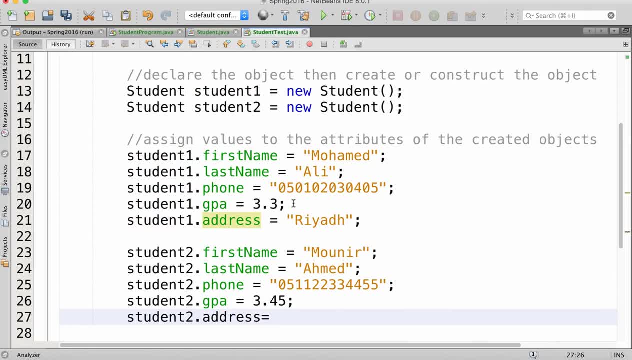 the objects will be updated with the new attribute you see now in terms of organization it it looks much better yes 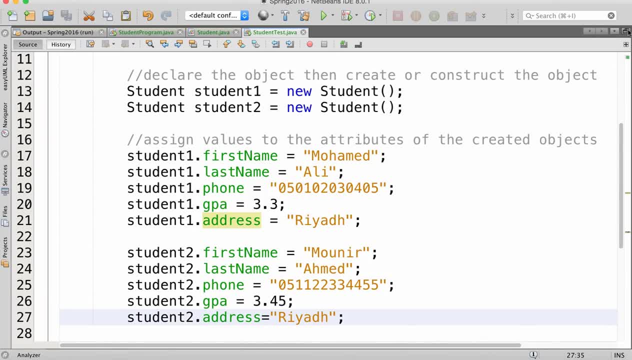 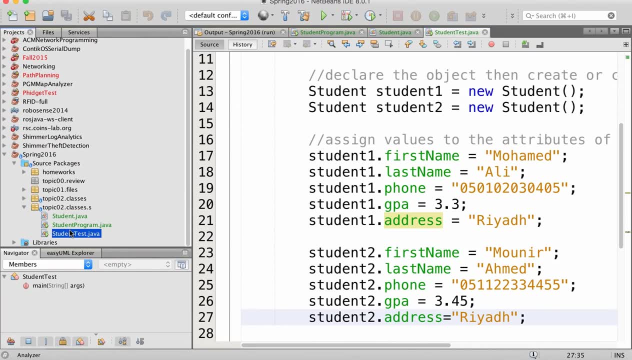 no it's because the class student is defined in the same package no it's because the class student is defined in the same package of the test so I don't need to import you import a class if it is not in the of the test so I don't need to import you import a class if it is not in the same package but this is the same package okay so I have access to all the 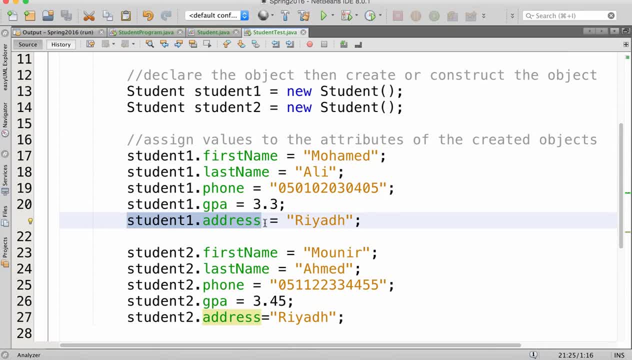 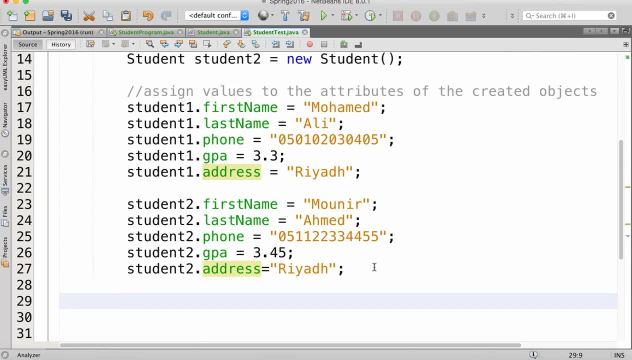 attributes of the class so this is the first improvement now if I would like to print I can do here s out print one by one but this is not efficient so as I 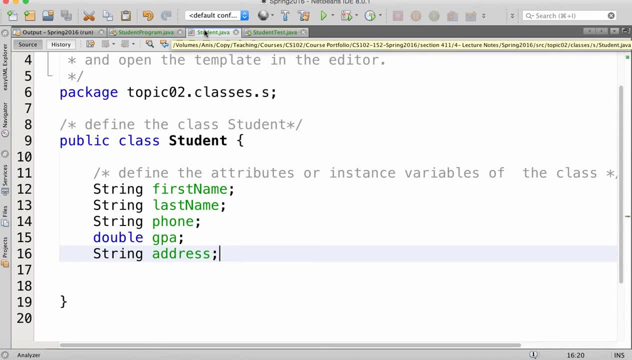 told you in a class we define two things the attributes and we already define this and the second thing are the methods it's exactly the same thing that you know in CS 101 the methods but now the methods will be part of the class characteristics usually methods they define operations on the class they define different types of operations that you can do on the attributes all that you can do in general the only difference with what you have seen in CS 101 is that in CS 101 most of the far all of the methods are defined as static we saw in CS 101 most of the far all of the methods are defined as static because rows want your unfortunately because it has a lot of in common with the other the transmitter a function which which allows and the only difference is that if you want you to see Yes 101 is the topic. in CS 101 which also smoother what you'll find in class and I'll be trying the class box but not because you do everything in one class 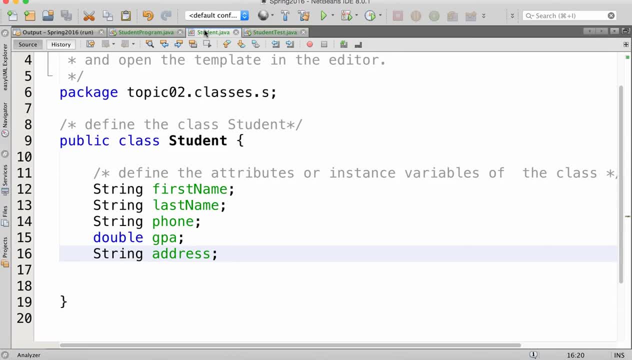 now we don't need to define them as static okay because they make part of of the class 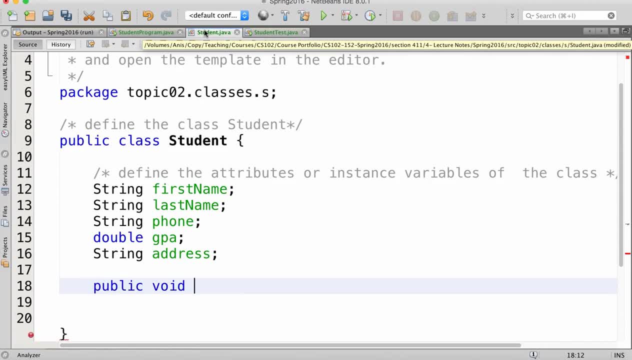 so here i'm going to declare a method which does not return anything and i'm going to call it print info 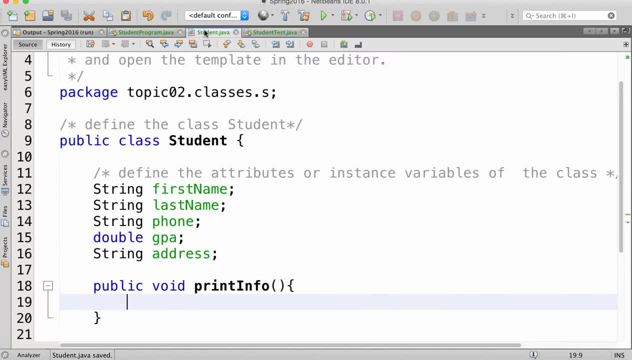 so print info is going to show all the attributes of a student just to make it faster i'm going to copy all of this and i will make the changes 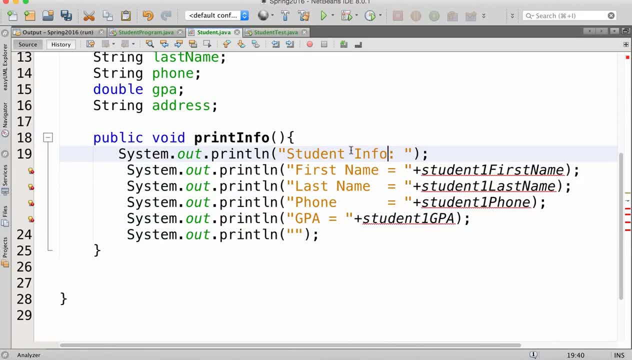 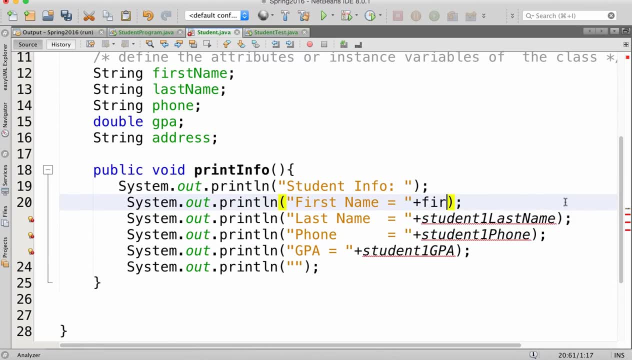 okay so student info what i should write here so i just need to write first name 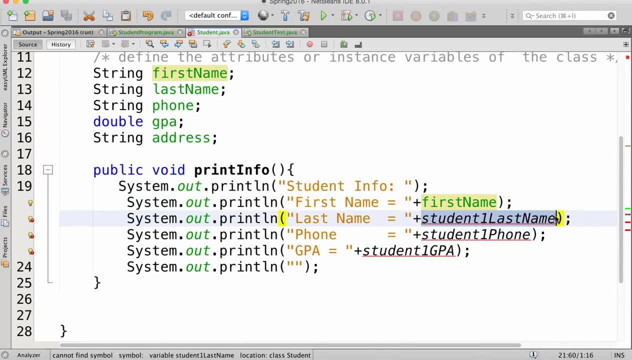 okay and here i write last name and here 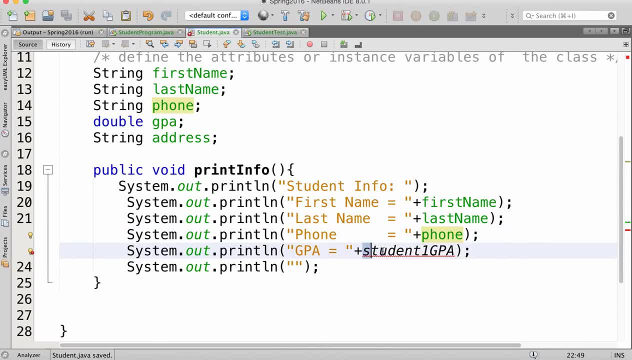 phone and here and here the gpa and i can add also the address i can the address here add the address here 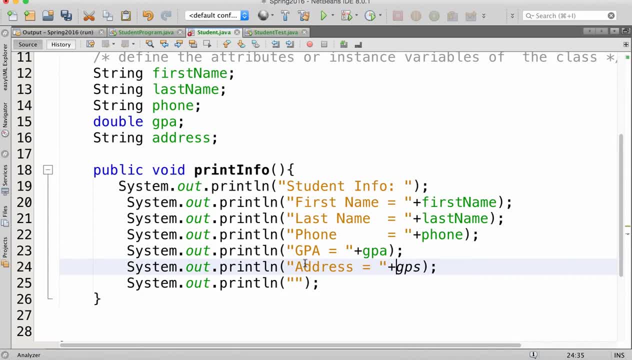 okay so i define this method yes sorry we don't need i will explain you i will explain but i will explain but i will explain you later not now okay 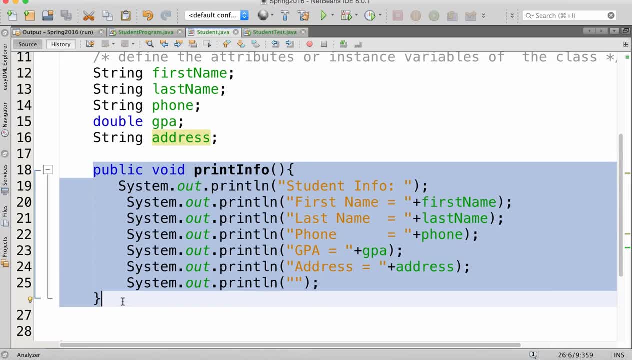 maybe in two lectures i will explain what static is because if i explain now it will not make too much sense for you 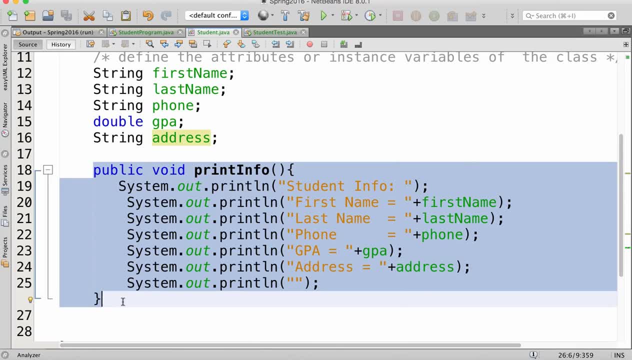 okay there is a difference between a method that belongs to a class and to an object so it's better to postpone this explanation for 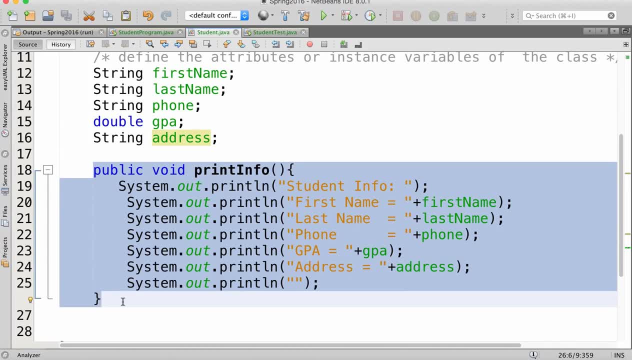 but now we don't need to define a static method 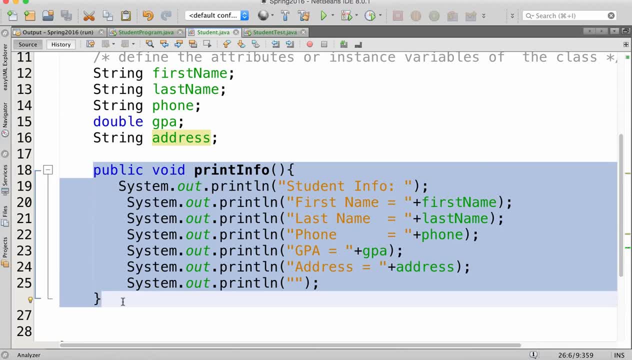 because the static method would have a different meaning later on if we are going to define okay 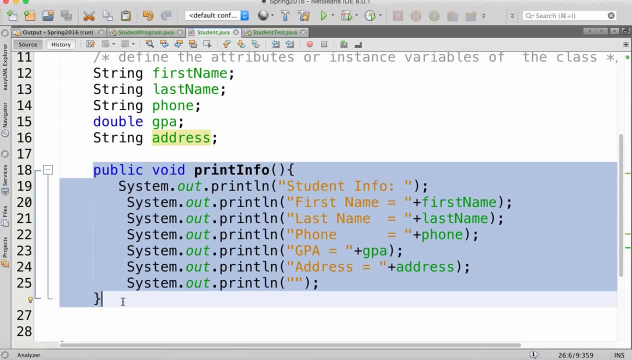 why do we create method? because you would like to do some operations on the attributes so methods are defined to make operations on the attributes here the operation is just 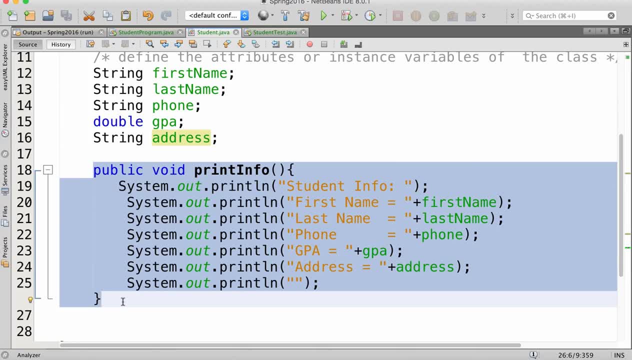 displaying I can for example make an operation changing the GPA increasing the GPA decreasing the GPA in the class yes now the advantage of defining a method 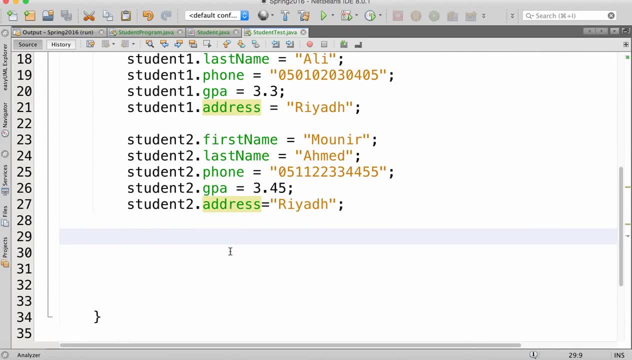 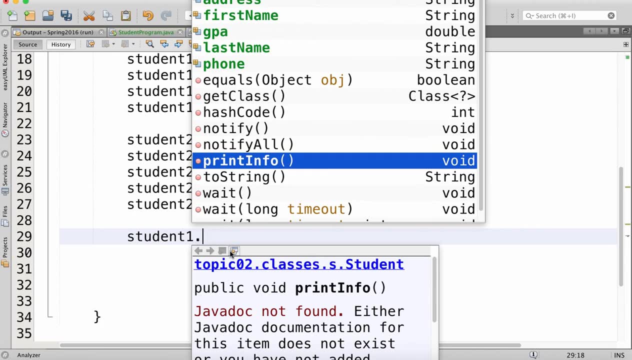 in the class is that if I go to my test program I type student one and I am happy to find print info I don't need to rewrite all these instructions and now I 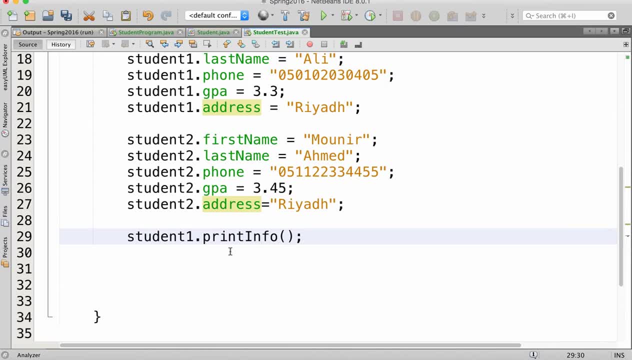 start to see that my code is going to be smaller if I don't have this method in the class I will have to write all these five or six lines and is going to make 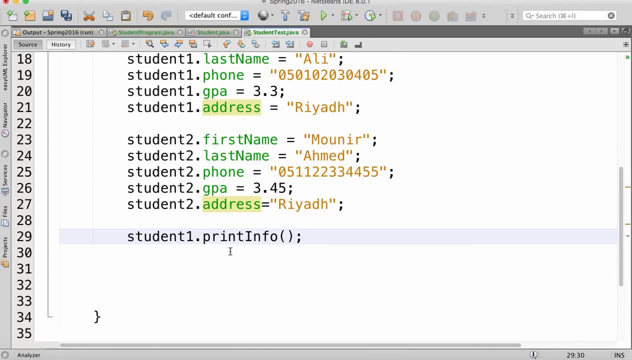 my code bigger right okay so I can also define student one student to dot print info and it's fine so now we start you 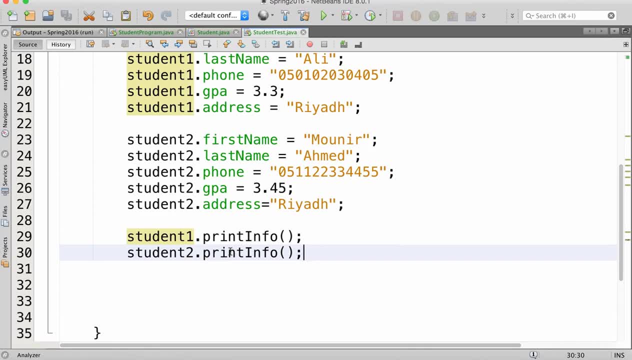 the first improvement in terms of reducing the code size and you will see even much better improvement in terms of reducing the code size so here we call it calling the methods of the class student okay or calling the method print 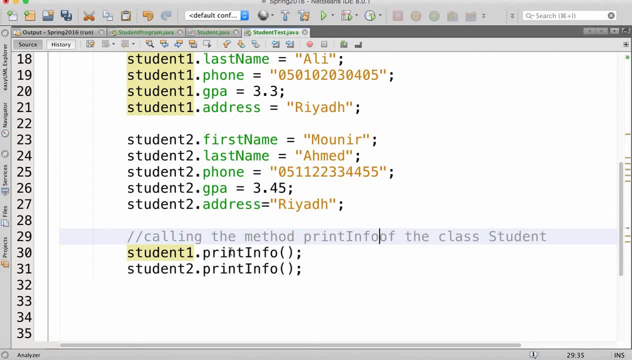 info of the class student so we call the method and this method is going to be excellent good 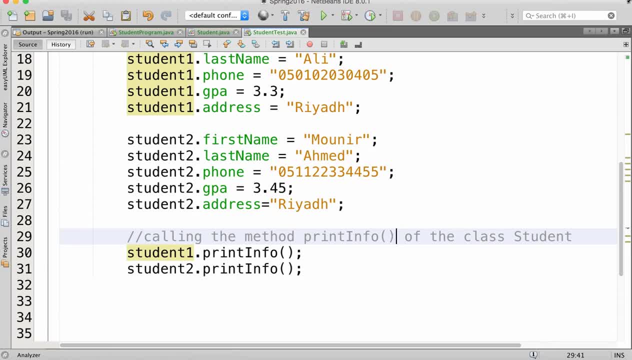 I can see the workload as far as what class in my test has to be executed is going to print the first name the last name and everything so if I execute now I 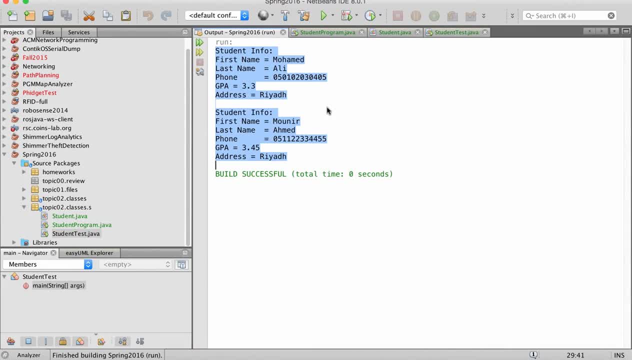 execute my test program I have exactly the same output as it is very long 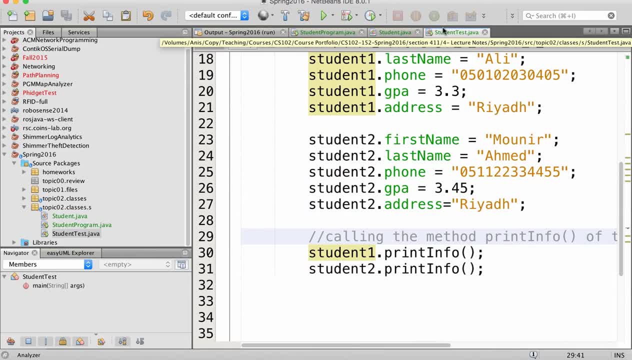 program okay but now what's the difference you know it's not a matter of writing the program that works I have it in the same program that works in two different ways but one of the ways is much better than the third and the second okay now I can get my code clear it is not a request but first I need to 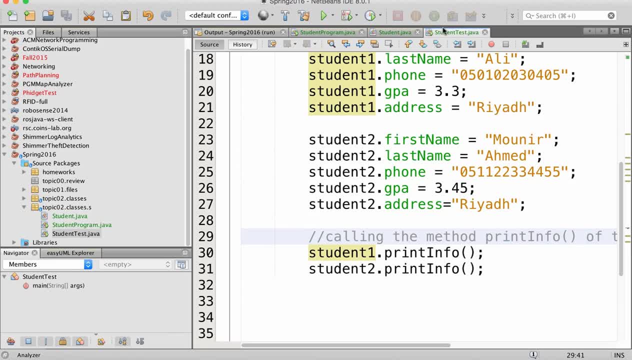 it's a matter of taste not not a matter of just making something that works okay this is an introduction to software design to software engineering to 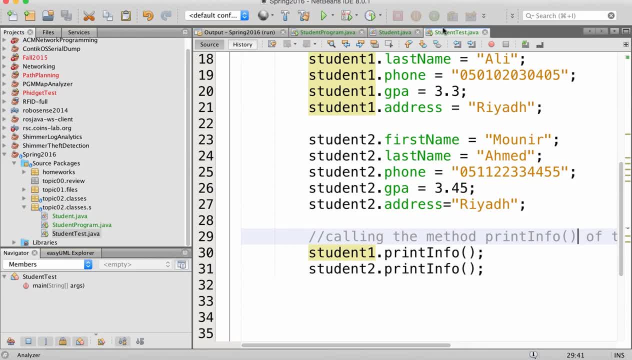 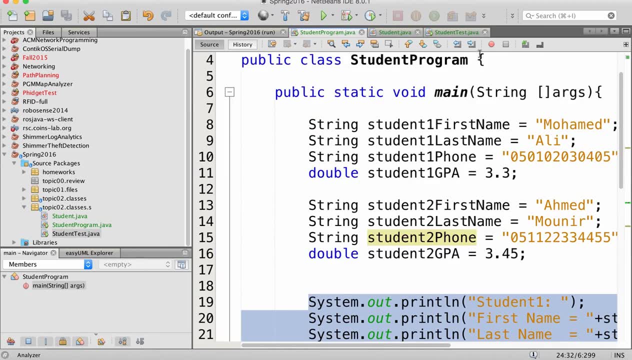 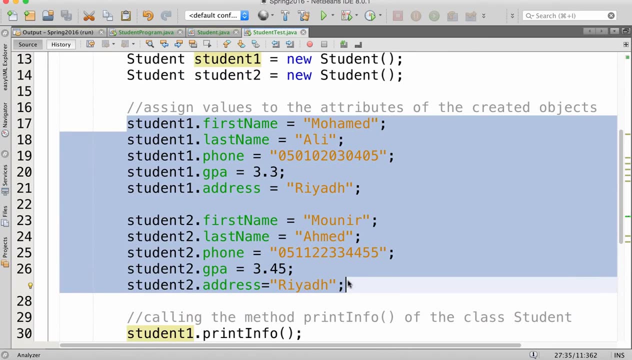 software development not just making simple programs that work okay excellent still I don't find these very fancy it takes me a lot of line codes you know one of the quality 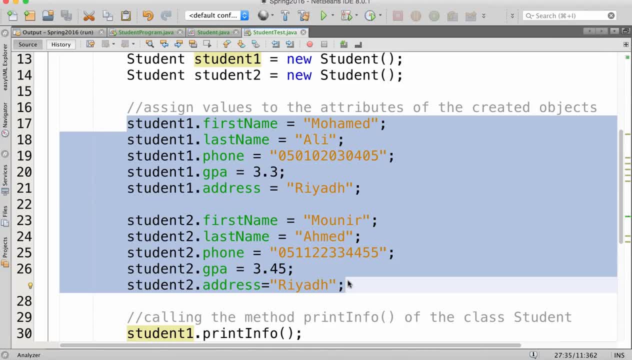 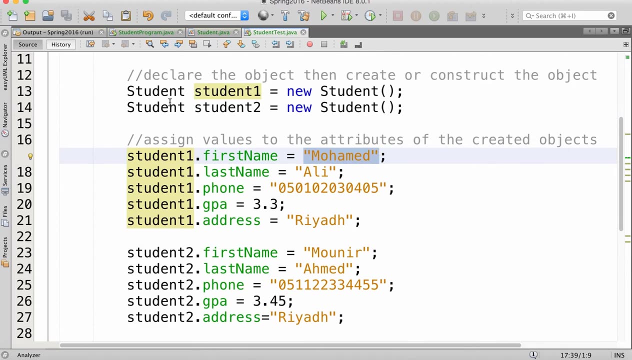 measures of software is that you reduce the code size as much as possible in general okay so I would like to reduce my code size so these values are initial values that I would like to set when I create the object so in what I did now I just created an empty object 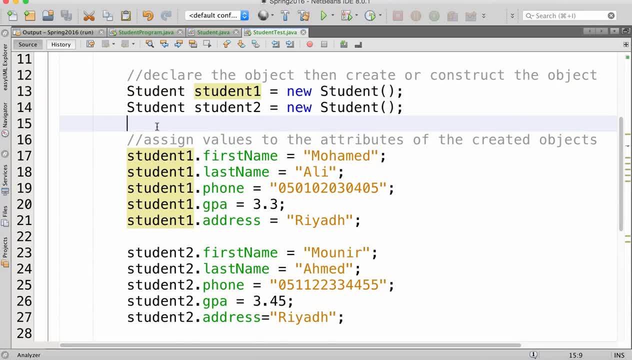 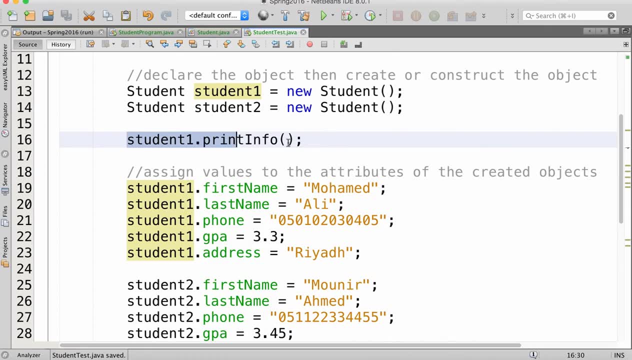 that does not contain anything so if I make student one dot print info here in the beginning 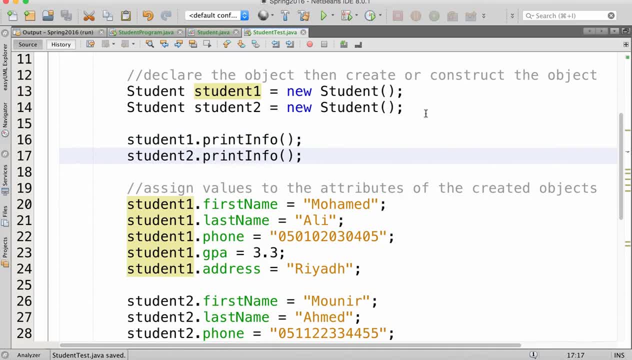 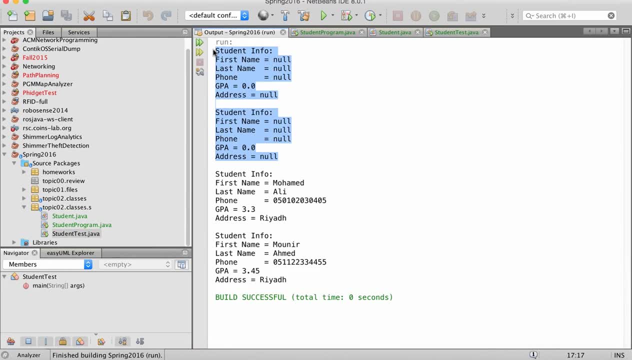 before before making any assignment the values are none and zeros okay and then after the assignment the values have changed 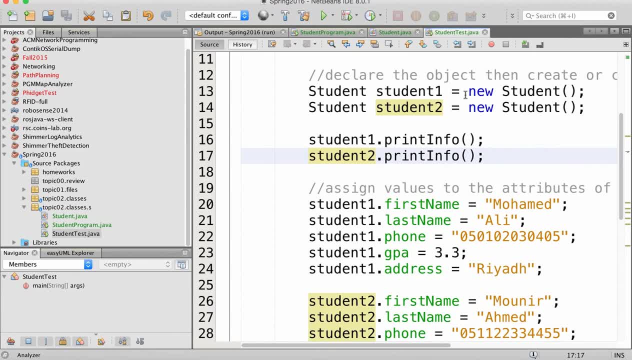 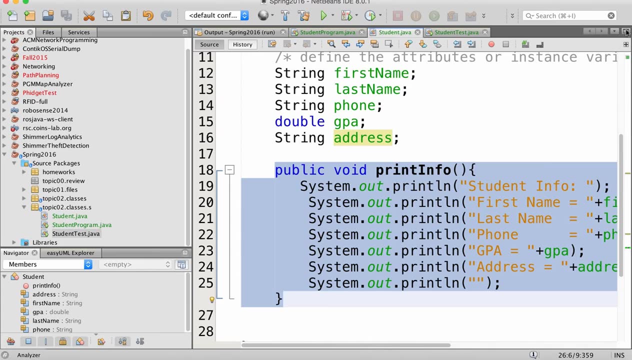 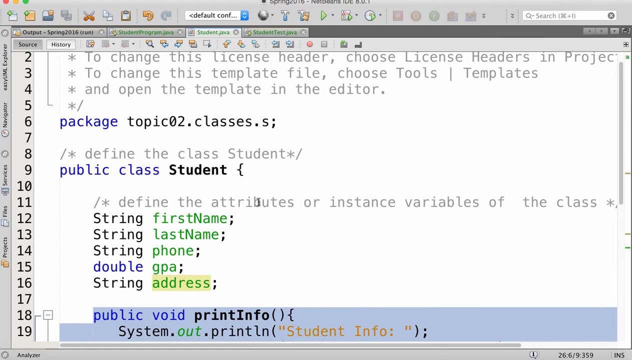 now I would like to make another improvement I want to initialize at the creation of this okay so this is possible in object-oriented programming by defining what we call a constructor so here in the student class I can define a special method it's a special method that is called the constructor 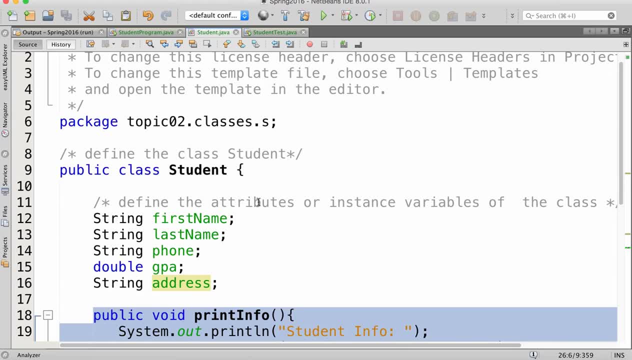 it's a method that constructs an object and what does it mean construct it will initialize the attributes to some default values okay so the 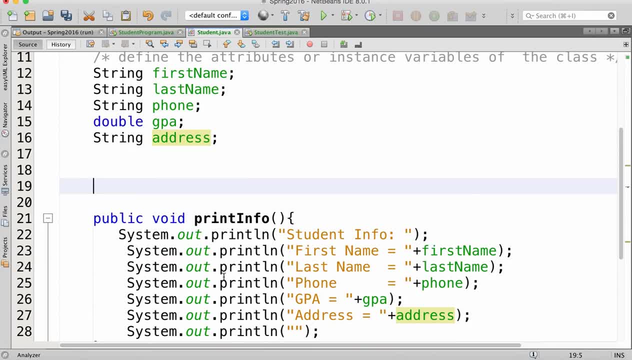 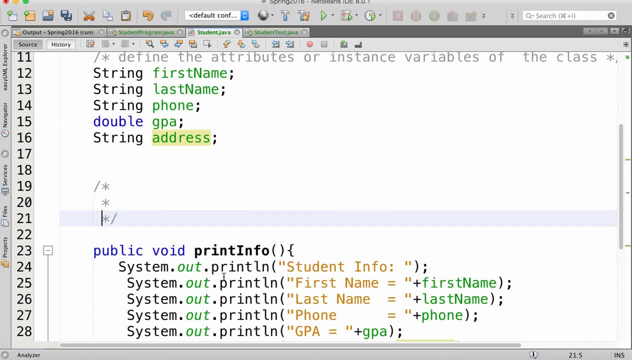 constructor before writing a constructor it has three attributes or it has three characteristics not attributes it has three characteristics the first characteristic it has the same name of the class let's see 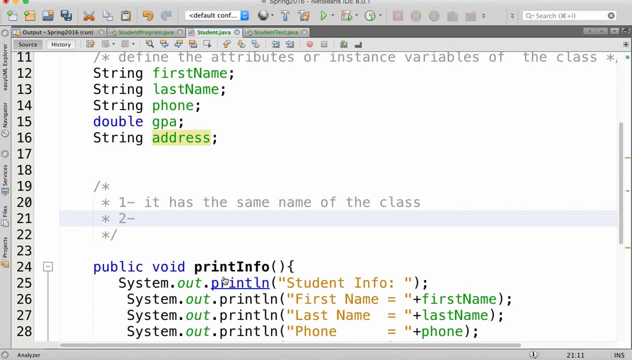 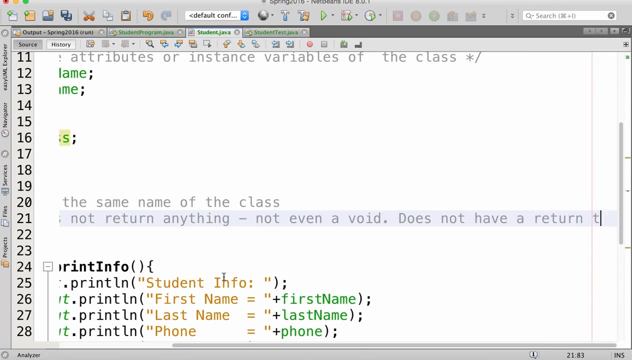 ok the second characteristic it does not return anything not even avoid or does not have a return type it does not have a return type ok this is probably more explicit ok 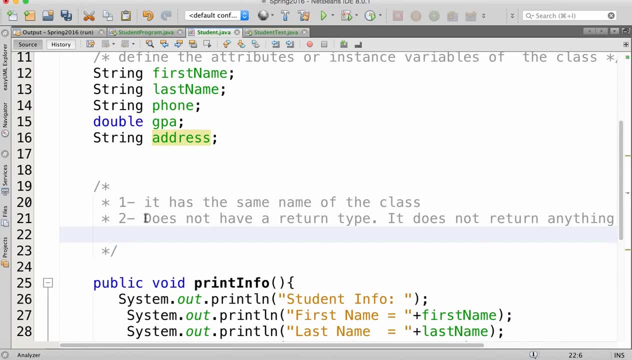 the third property here it must be declared as public we will see some 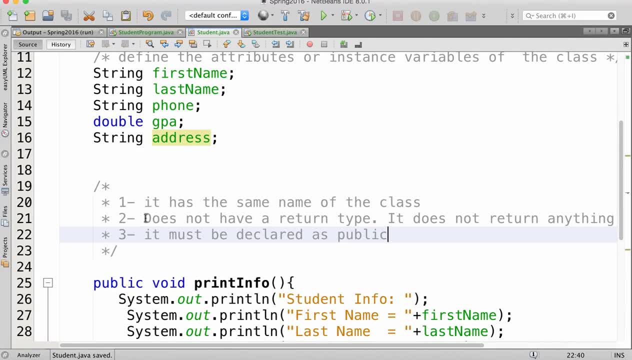 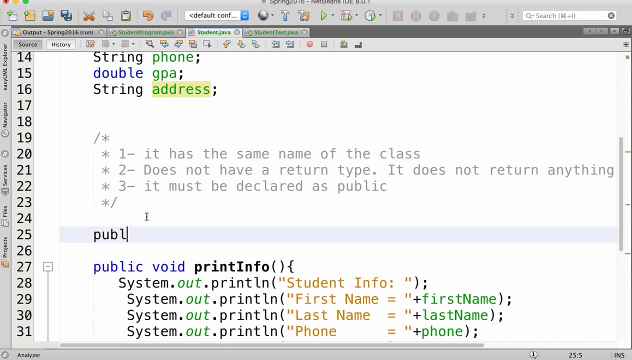 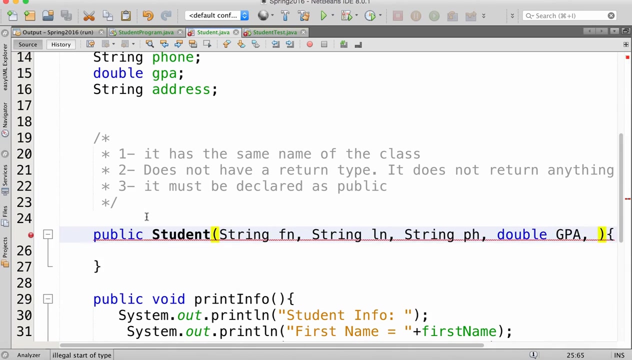 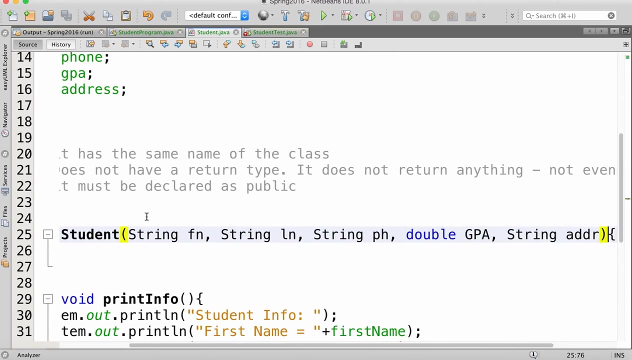 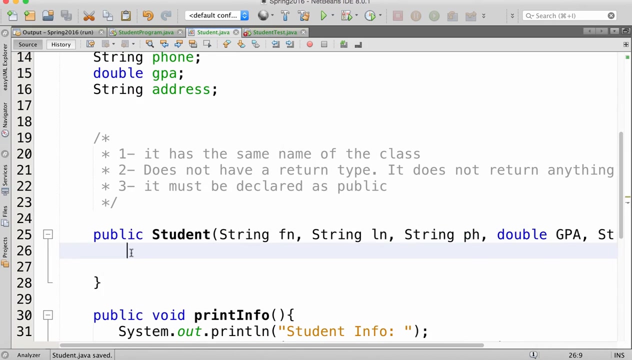 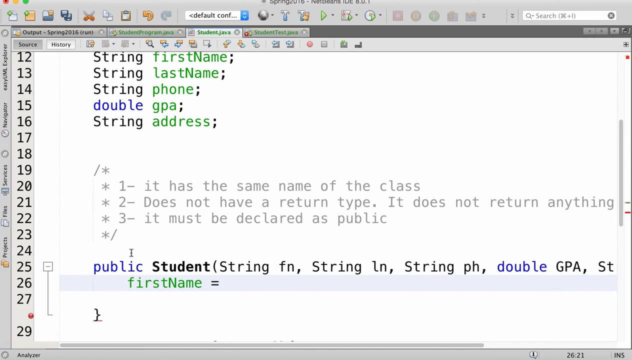 exceptions when we go more advanced but 99.99% the constructor must be declared as public so to be visible from the outside to be able to create now I'm going to apply these rules so what should be my constructor it should be first public it has the same name of the class I will apply this student okay it's a method so so this is a constructor but now I would like to define a constructor that provides some default values so I will put the default values into the attributes into the parameters the list of constructors so I will put the default values into the attributes into the parameters so for example here i'm going to use fn for the first name and then string and n for the last name and then string ph for the phone and then double for gpa here with capital letter and then another string for address addr and i will use this list of parameters to initialize to give default values to the attribute what is my attribute name first name it will be equal to what to gpa 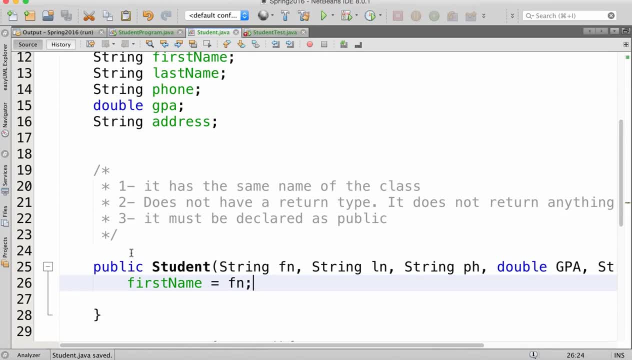 to the parameter fn so i make an assignment now i assign fn to the first name same thing last name fn equal and then ph equal phone correct no sometimes i see this error it's not that in common but it's an error we should assign the parameter to the attribute ok so phone equal ph 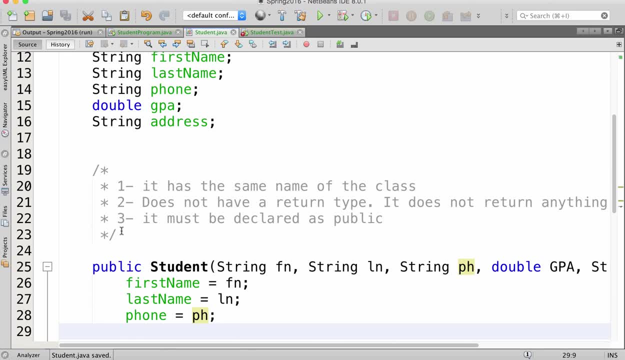 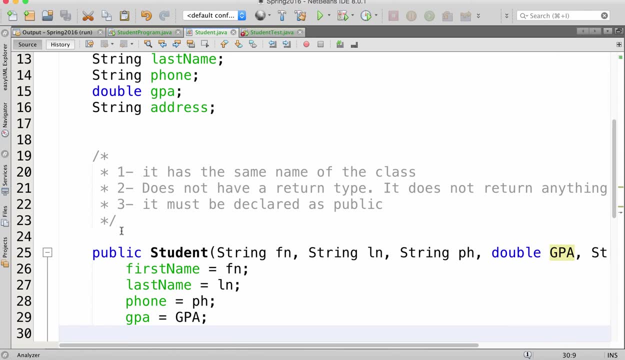 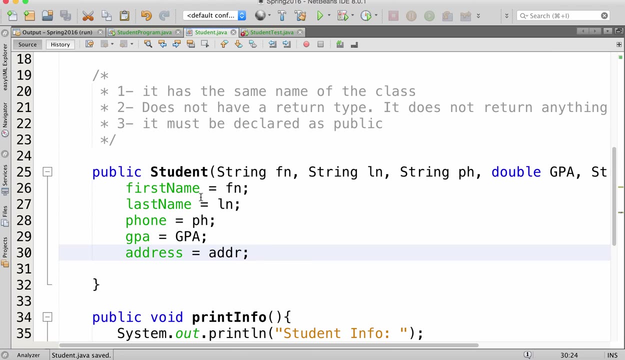 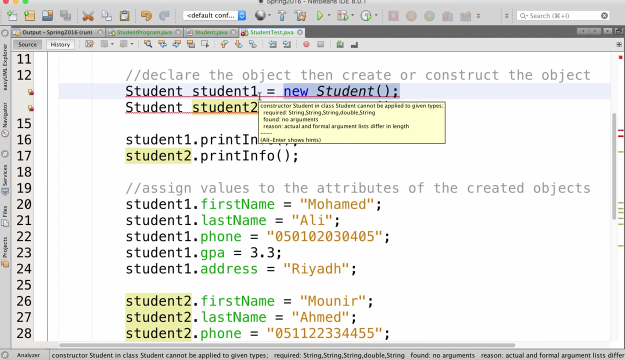 and then capital or the ok equal capital and then address equal addr so now i have a constructor with some parameters ok how can i use this i will go to my class and 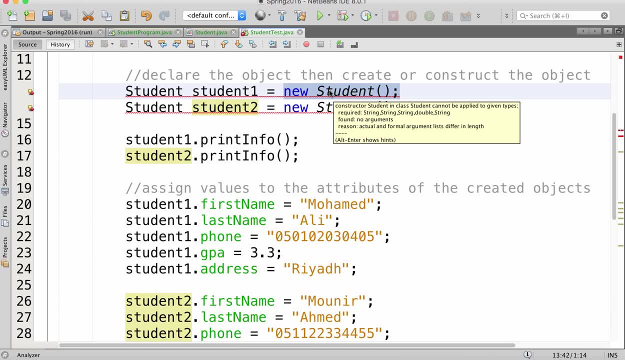 unfortunately now i find something unpleasant that the code that was working before it's no longer working so i'm going to go to my class and i'm going to go to my class and i'm going to 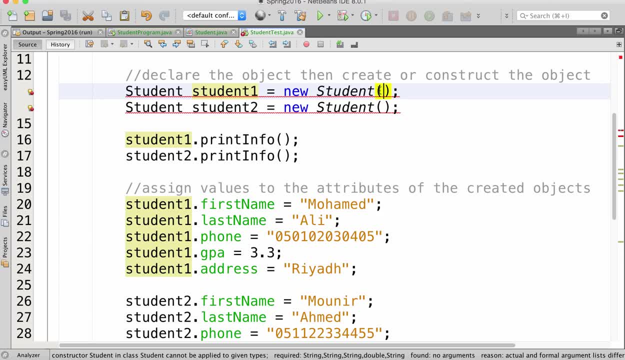 go to my class and i'm going to say hopefully it's no longer working 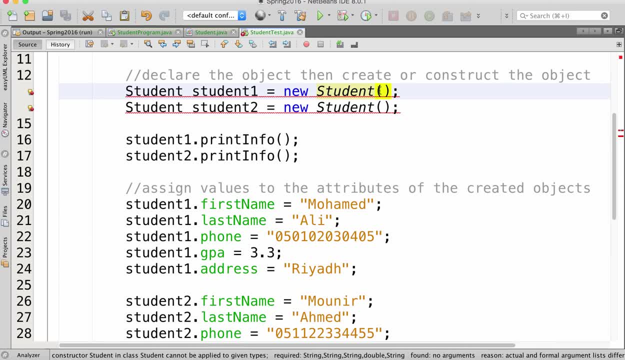 ok so we can guess why we need to provide some parameters here so obviously first of all we need to preserve the order look now the order first name last name phone if you do a phone number at the first one it's not going to be wrong it's going to be assigned to to the first name so i'm going to put here so 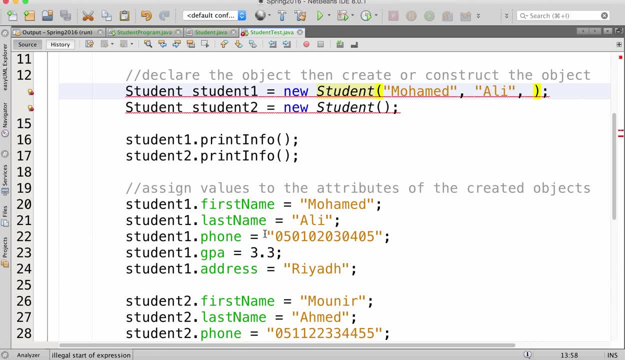 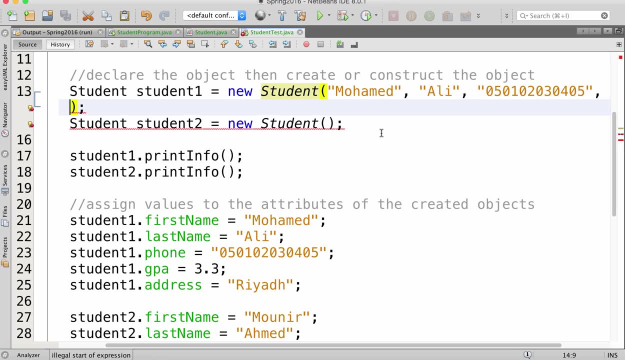 last name phone number and then we got three and then the address is there any 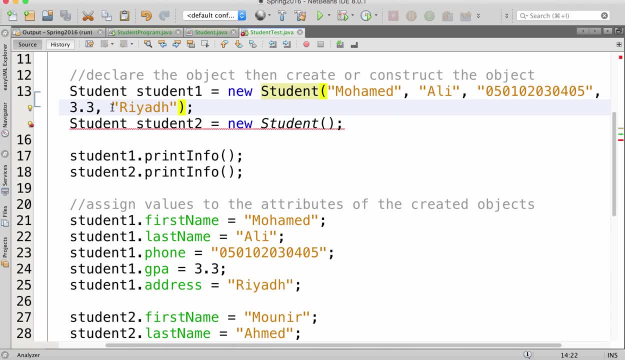 competition error for student one because now we have used the constructor that we have defined but now for student two it doesn't work 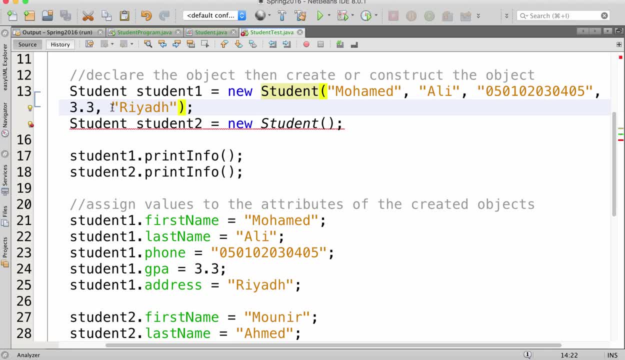 why it was working before and now it's not working but before it was working 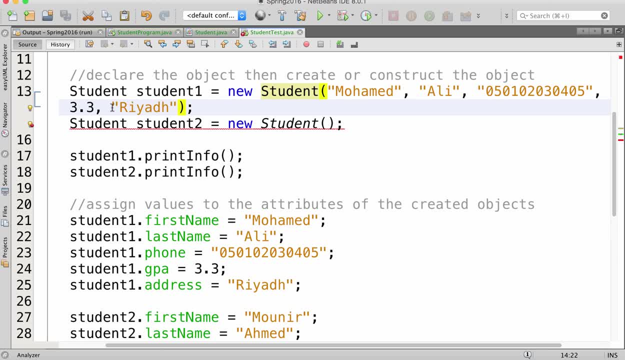 but man yeah the same class but before now if I remove this the population error change if I put it back what does this mean so this means if you don't define your 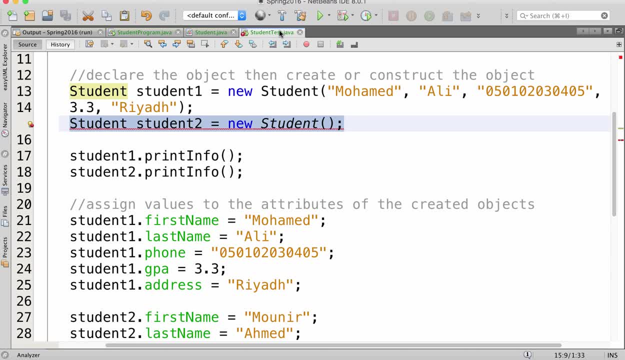 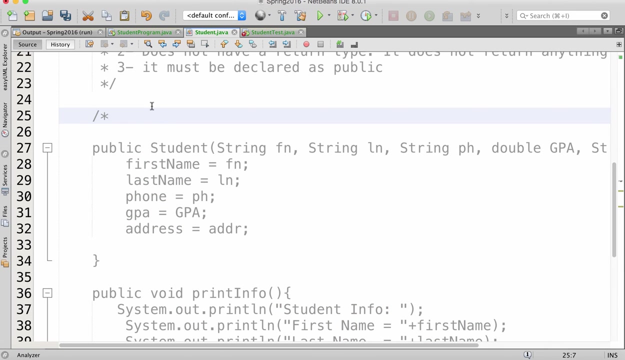 default constructor okay the default constructor is a default constructor that initialize everything to default to null and zeros so this is automatically provided by Java if you don't define your own constructor if you define your own constructor it means you have overridden this one it's no longer used and defined and so that now for the compiler it's not defined so you have to waste either you don't use a default constructor you use only the constructor that you have defined or you can define a default constructor that's what we are going to do I'm going to be fine default constructor and I use the 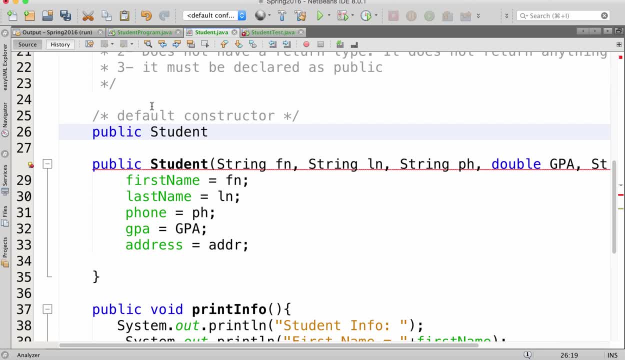 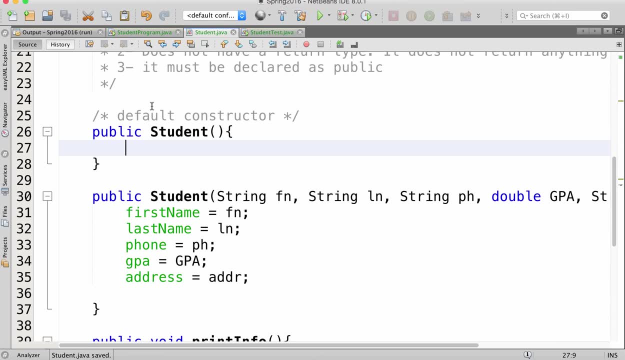 same rules public name the class and the default constructor does not have any parameter so now if I 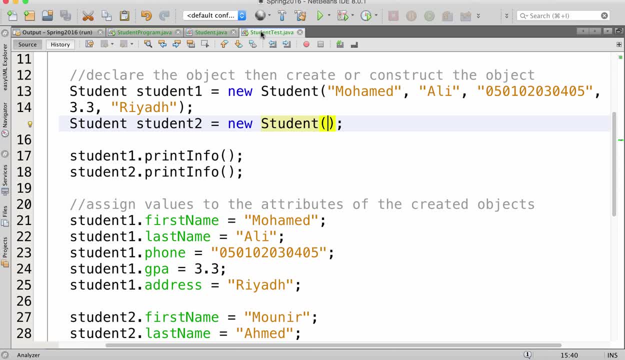 go to student test it's getting back 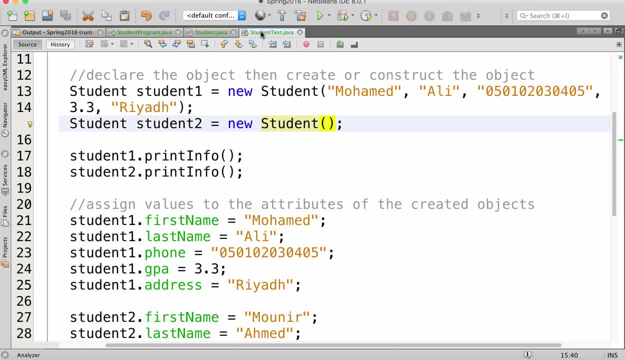 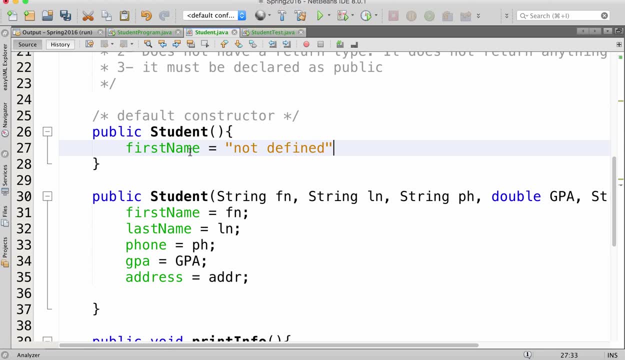 because now I have defined the default constructor so you have options you can do for example first name is equal for example to not defined that's possible and to initialize to some static values but it's more common to put the default constructor as not doesn't do anything so everything will be put to null and zero yes we can do this I'm going to show you that later stage we can define 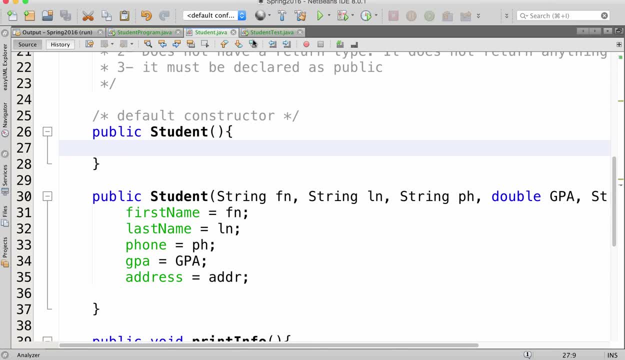 indeed several constructors but now let's apply okay 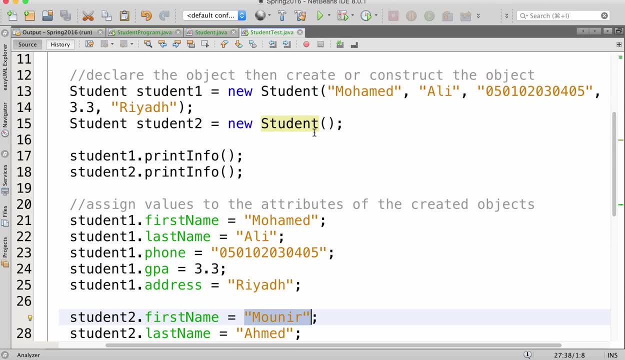 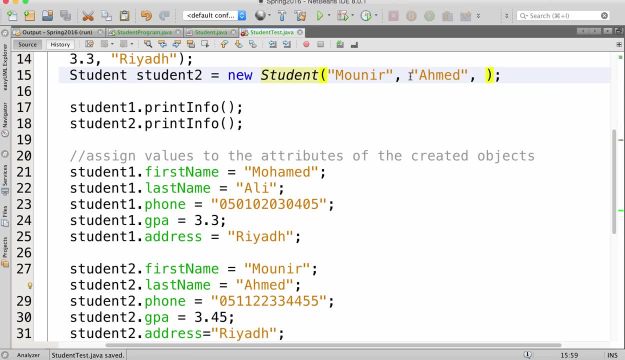 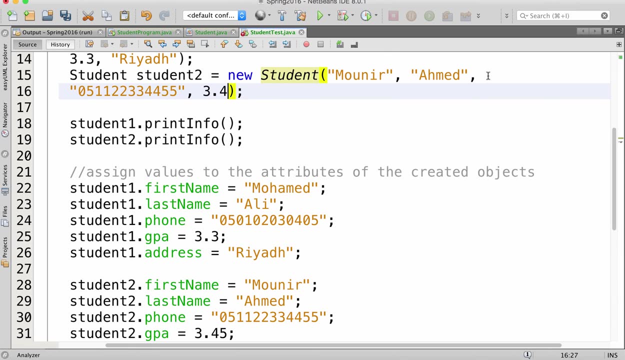 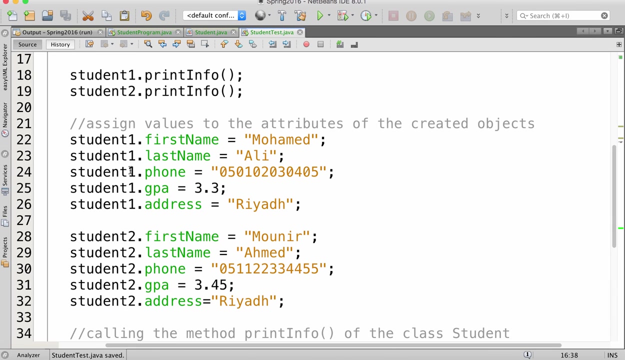 so I have two constructors but I'm going to still to use the argument constructor the constructor with arguments okay so I need to copy all of these parameters here so do I still need these values so this will not make part of 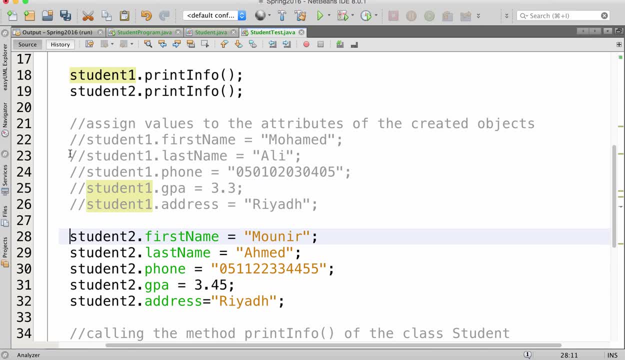 my code anymore look how much line I have saved now is it better look now I'm 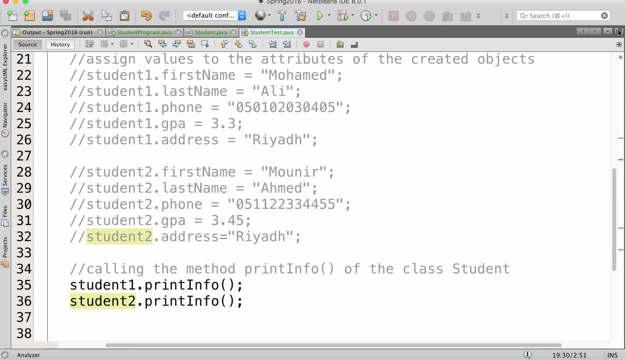 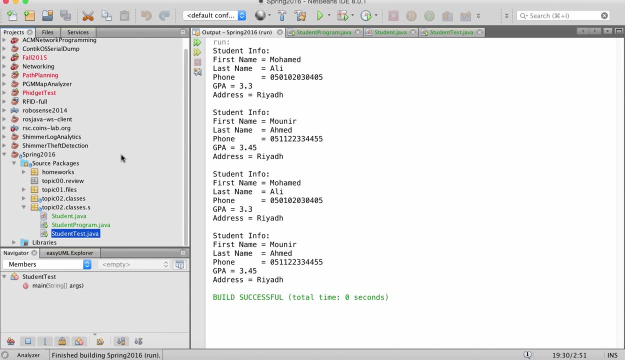 going to print print info twice so it's going to be now assigned from the very beginning so the constructor assigns the default values to my object you 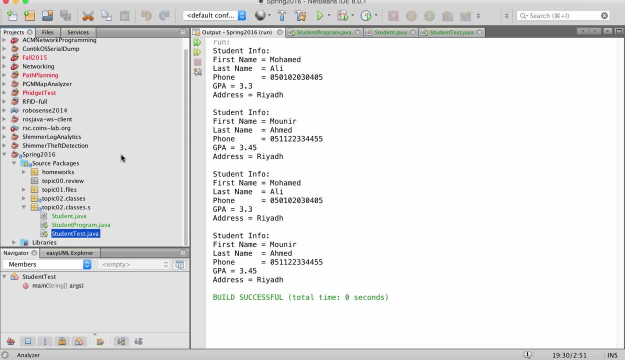 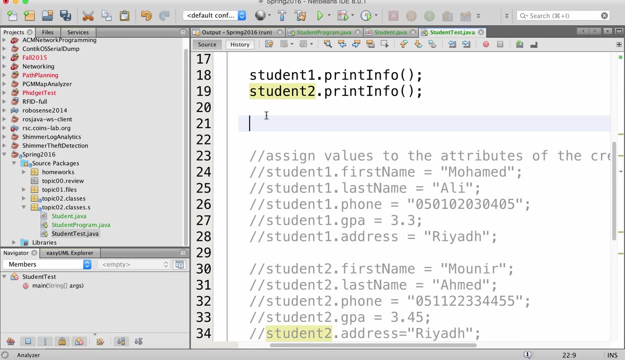 in the previous version it was null and then after assignments we get it to the default values and now since we have initialized the attributes in the beginning it was working fine okay so this code not even this look now I'm going to 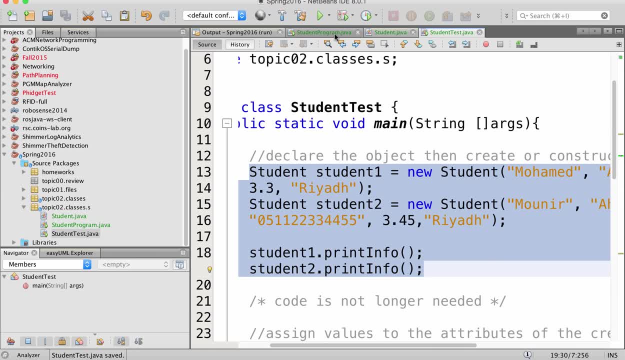 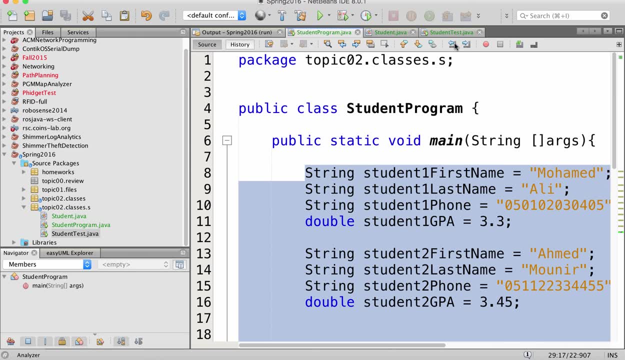 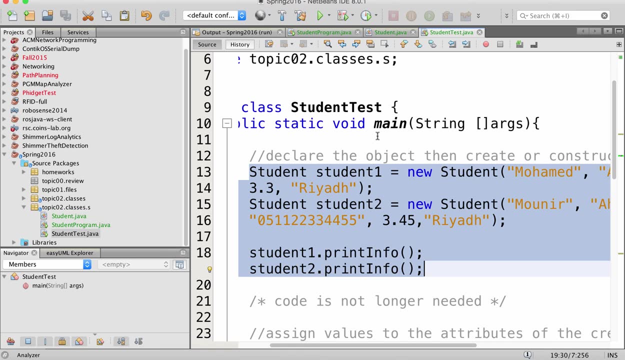 create this code for the array of line with the constructor and this is our new thing right here we have four lines of codes as compared to thirty lines of course 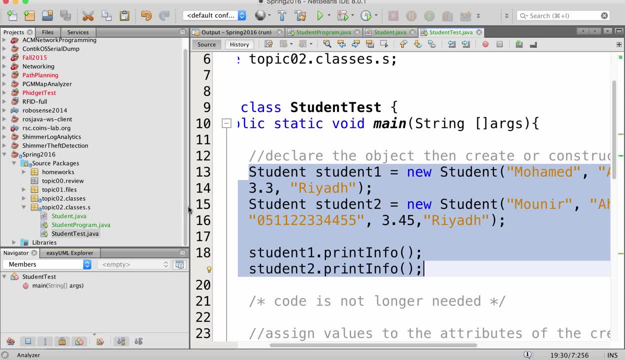 sorry yes yes you will see this okay so what is better now using classes or without yeah obviously 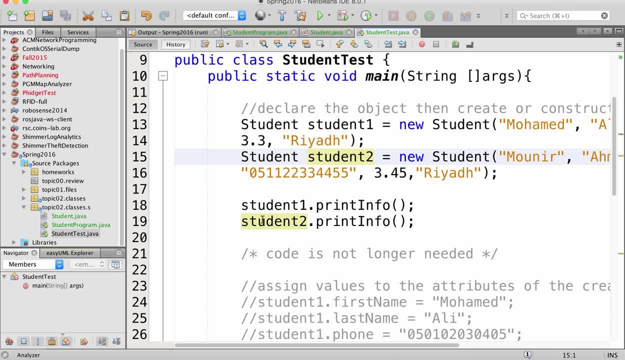 ok so so this is now an introduction to object-oriented programming to classes so now I think I understood why classes are important and how they had a lot to reduce the code size imagine that we don't use classes now these are only with two students imagine that they would like to use 20 students now if you 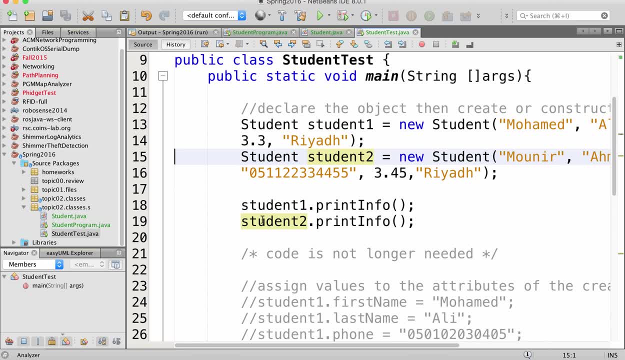 are going to use it in the previous way now you have to define them manually 20 students multiplied by five variables 100 variables just to define 20 students here I don't need to do so ok how we can define 20 students here ok 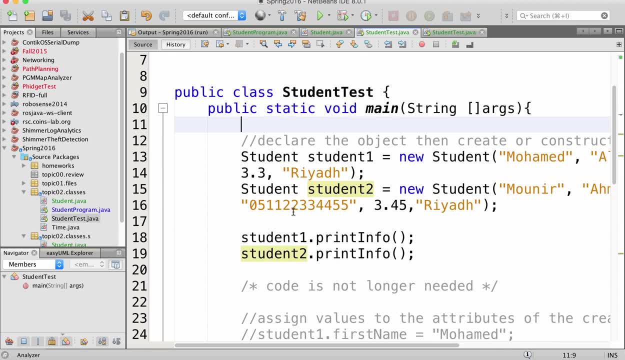 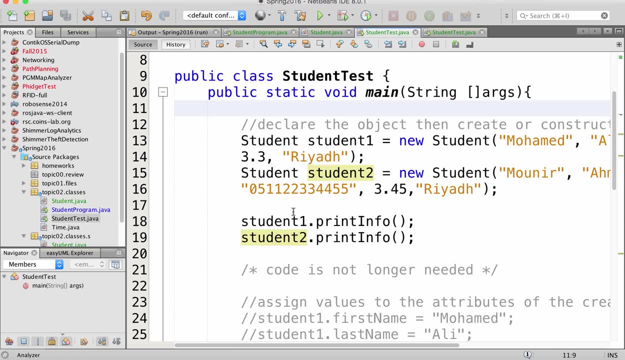 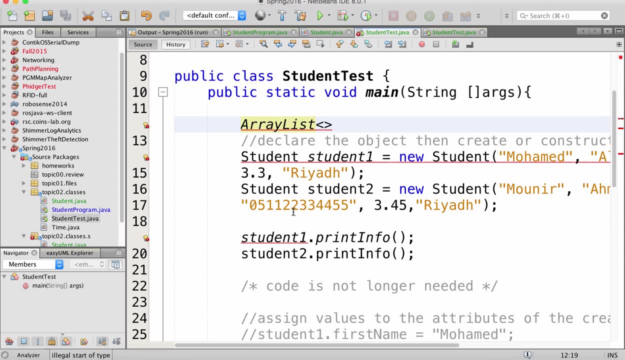 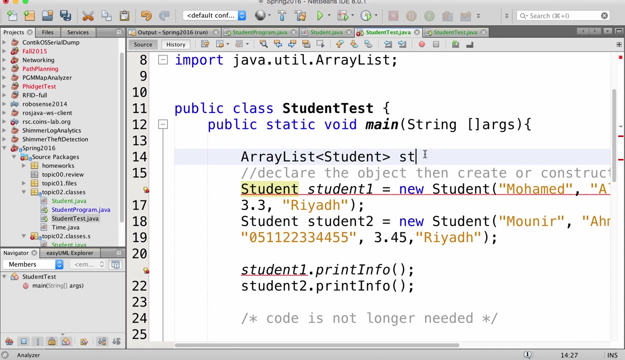 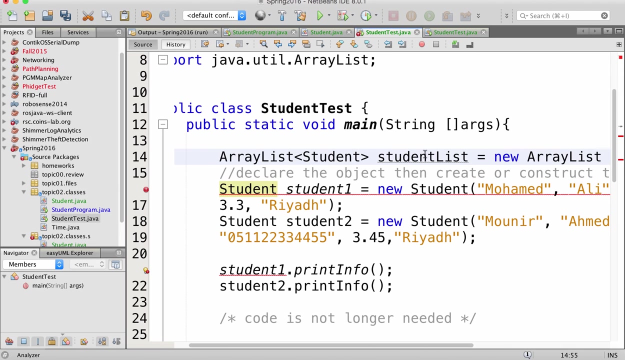 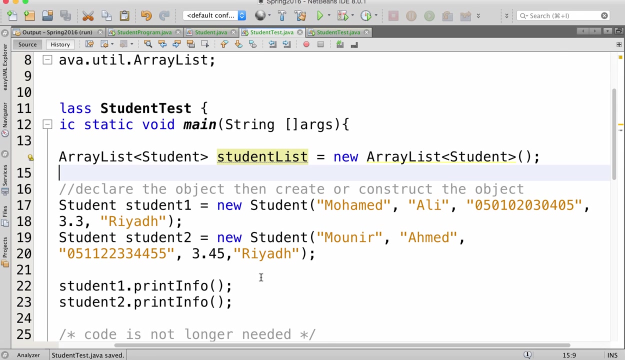 so I can't define an array list here ok it will be an array list of what of string ok imagine that we do it string what are you going to put in the array list the first name or the last name or the phone number all that the student is not a string a student is an object different from a string Saho Allah so I would like to create an array list that will store students because an array list can store string can store integers can store double and can store any kind of object so nothing bad if I just put array list of of student and I can call it student list which means that it 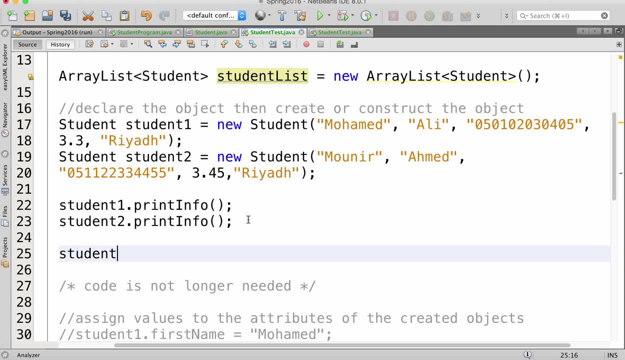 adds a name and it will add a string or it will give students so take string well these and then add a few adding all the numbers the first primary explains is adding all these 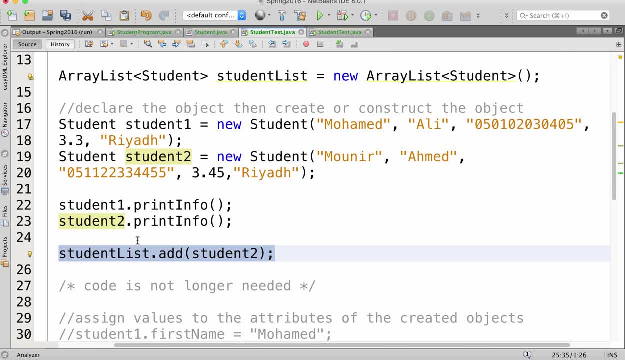 legible yes let's do this oh my goodness 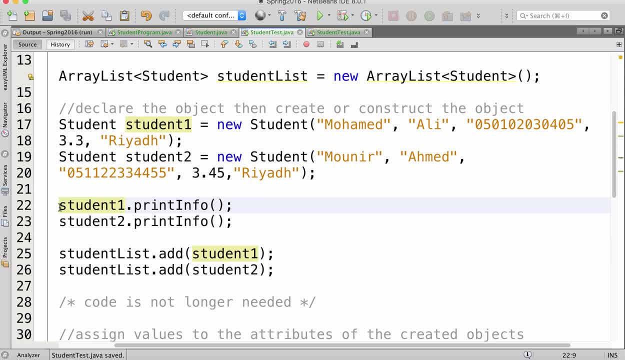 so if I want to treat now instead of treating one by one we can do what can 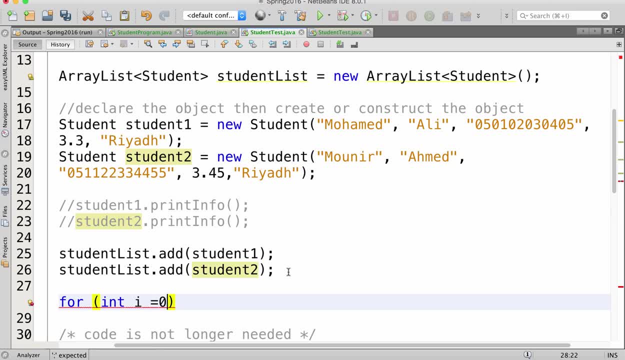 make a for loop for int I equal to 0 yes I less than my list dot size and then I plus plus 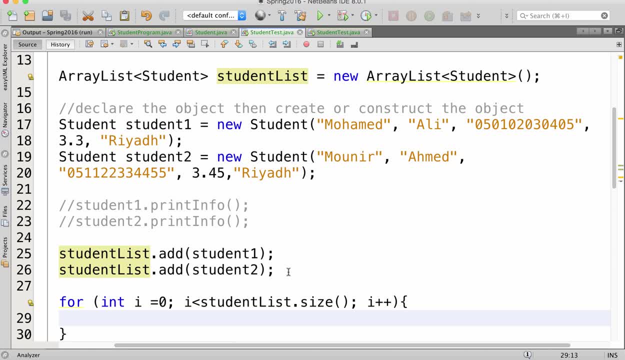 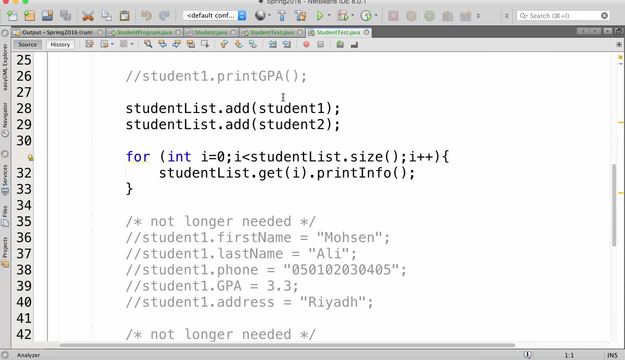 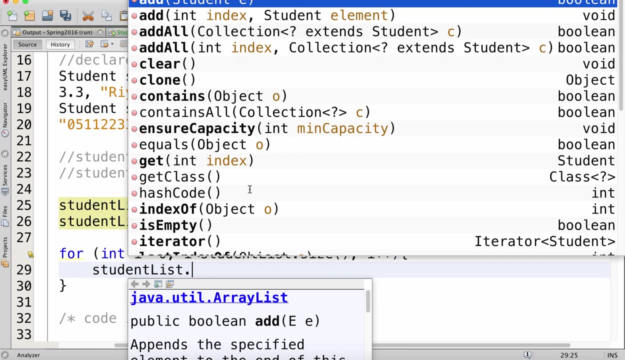 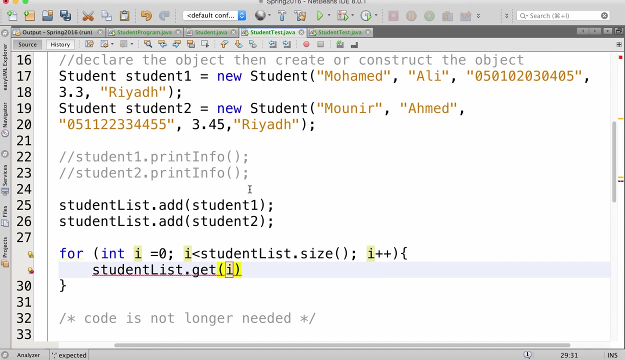 okay I want to print the student okay I want to bring the student now like okay yeah so student list dot okay so get I it will first return the first student and then we return so get I this is a student now if I want to access to the parameter or to the methods of the student I have to add another dot and they will get all of this so what I 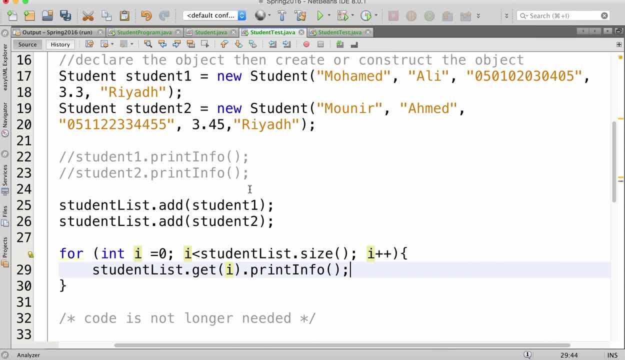 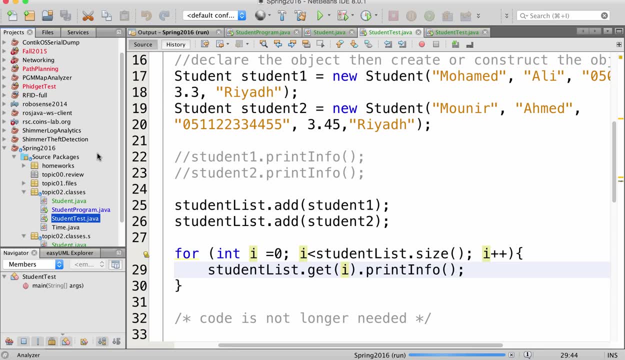 would like to do print info so now if I execute my code I'll get the same now even if I define 100 student it's not a problem for me if I want to define for them here I think the mission will become really very hard 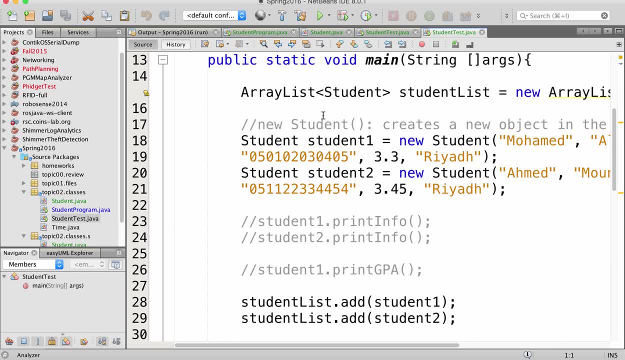 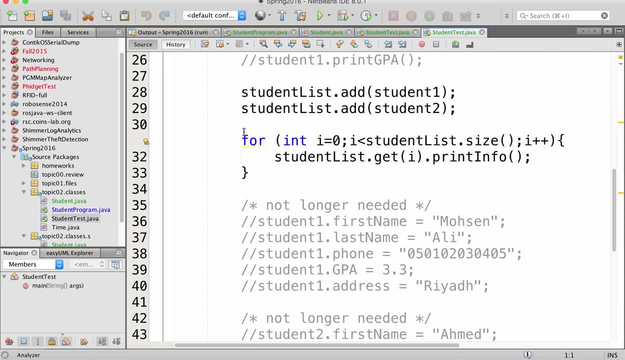 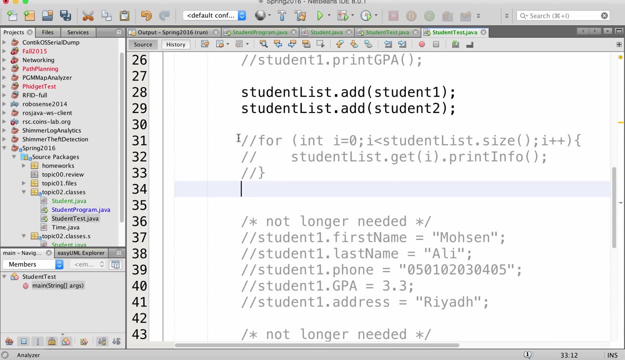 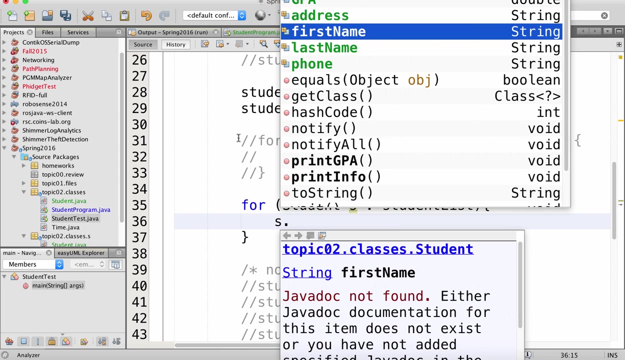 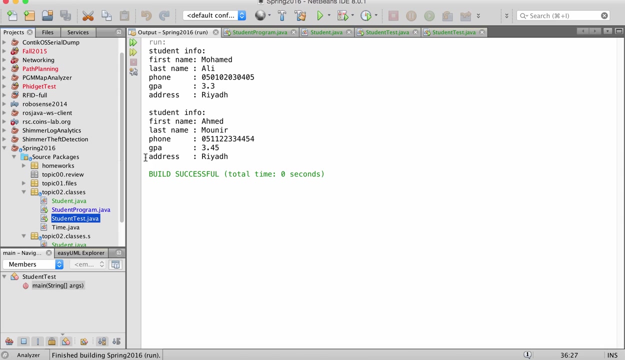 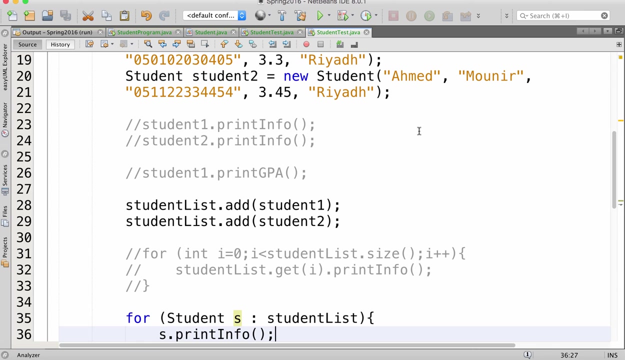 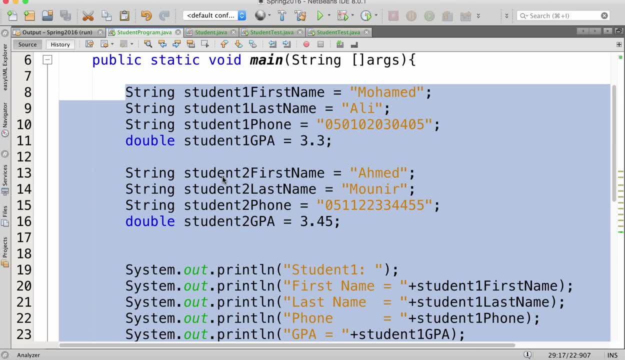 case is when we did everything with independent variables okay so that's fine for today this was an introduction to class and objects and tomorrow we are going to continue with more sophisticated features and efficient usage of classes and objects thank you